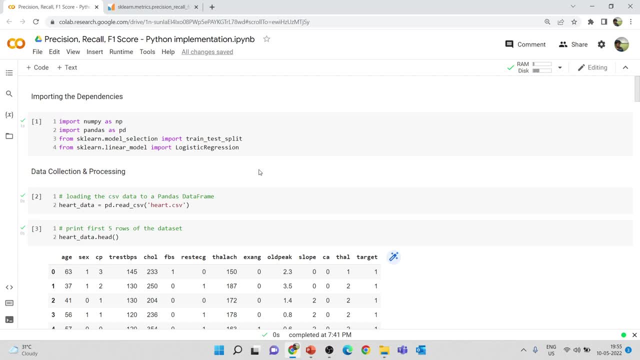 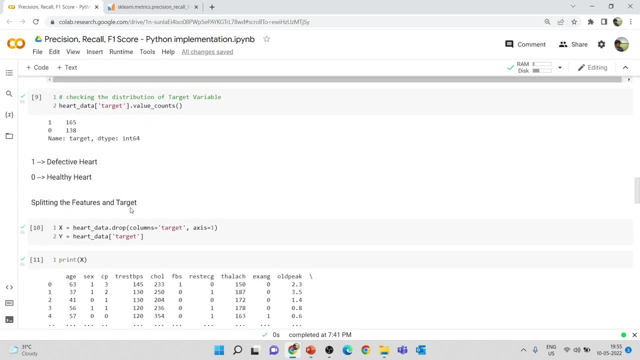 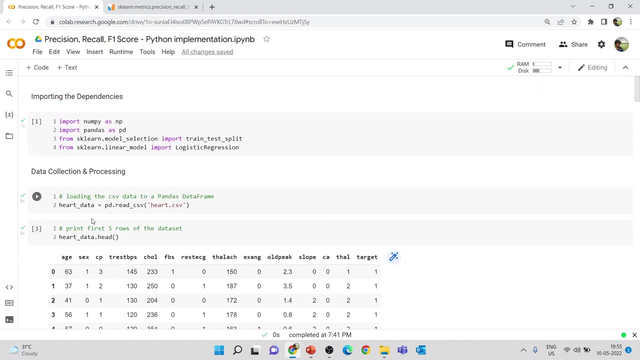 already posted video on predicting whether a person has art disease or not based on this data set that we have worked on. You can see here. So one here represents people with art disease and zero represents people who doesn't have any art disease. So this is what we have worked on. So if you want a detailed explanation on all the data, 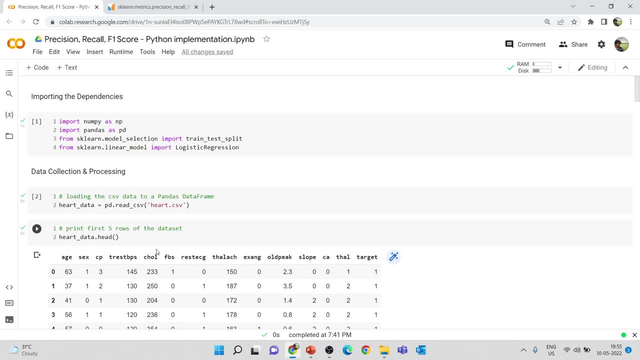 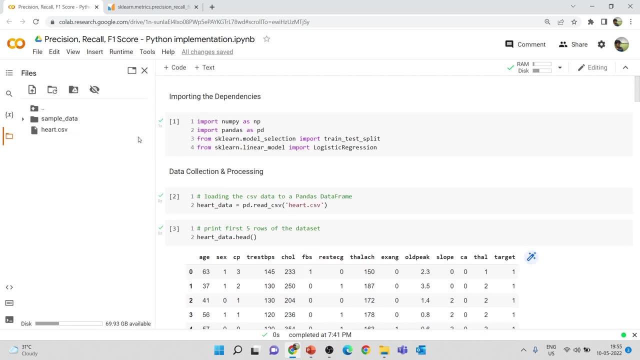 processing parts and how we are training the model and all those things. So I will give the link of that particular video in this video description. You can check that out. Okay, So here I have uploaded this artcsv, which is my data set file. I will also give. 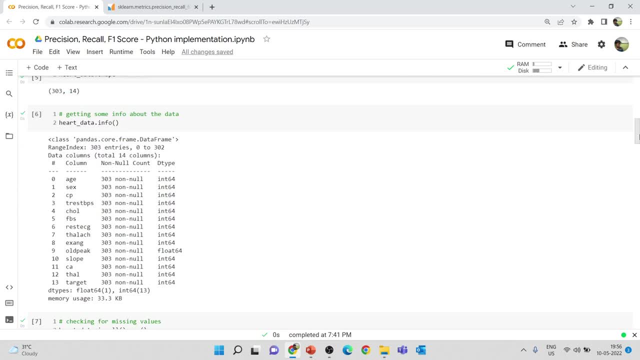 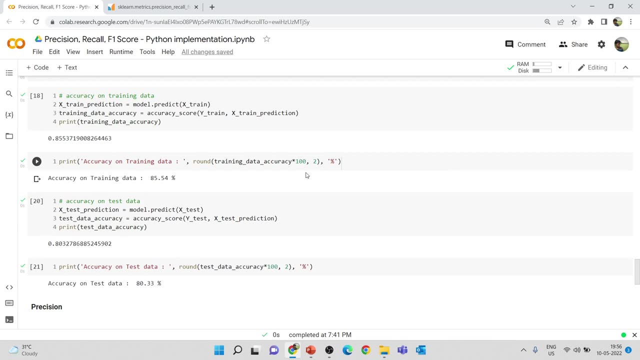 the link for this data set file. So in the last video- so like before this precision, I have explained you in detail about this accuracy score and you know how we can find this accuracy score for training data and test data and so on. So this is the accuracy. 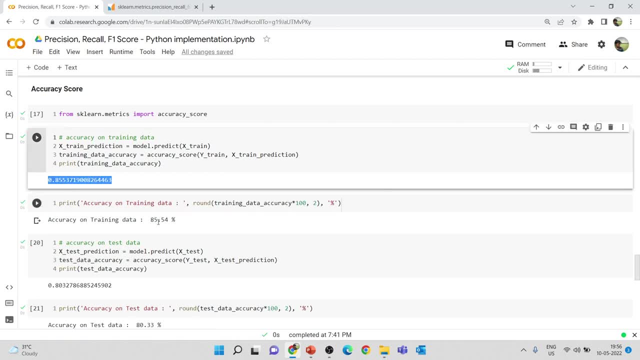 score we have, which is 0.85, which basically means 85 percentage. So 85 percentage means so, out of 100 predictions your model can predict you know 85 correct data points. So that's what accuracy means, and we have also discussed that there are some limitations to this accuracy. 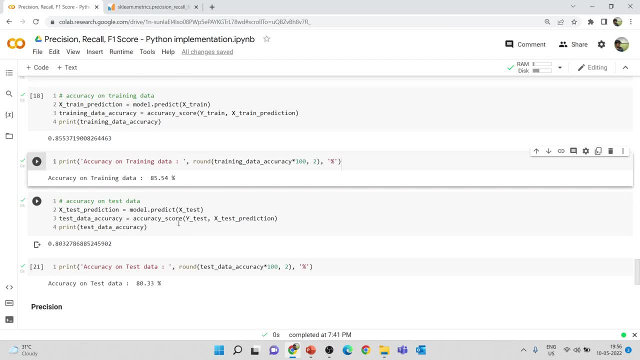 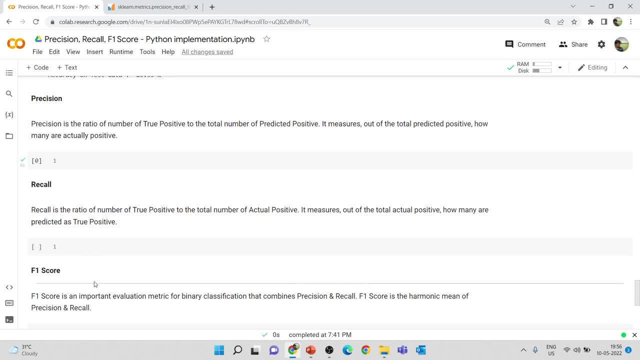 you know, focusing on the metrics such as precision, recall and F1 score, So where we have, you know, understood the other advantages that we can get from using these metrics. So if you haven't watched the previous video, I suggest please watch those things. So, in that case, only you. 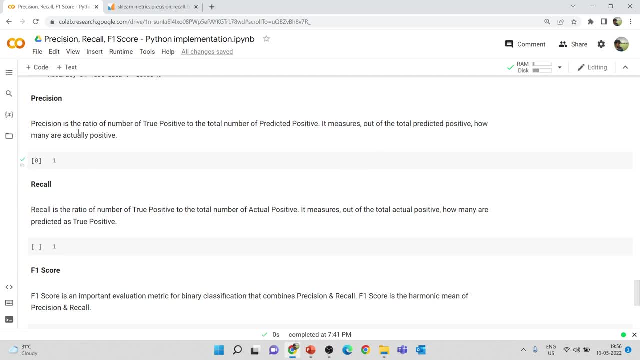 can understand this clearly. So this is the definition for this precision. So it is basically the ratio of true positive to the total number of predicted positive. Okay, So true positive means: so in our data set there are people with RDCs. So in our data set there are people. 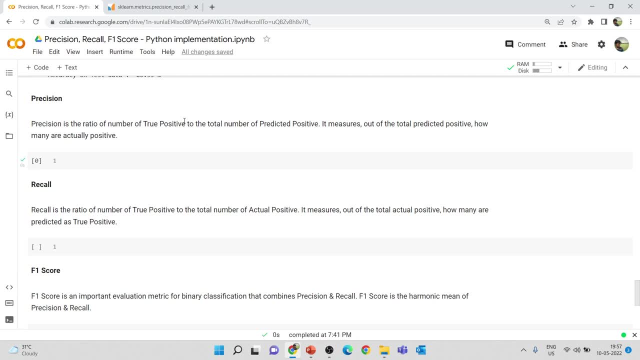 and without our disease, right? so true positive basically tells you how many people are, you know, predicted, as you know, people with our disease and they actually have our disease. okay, so here the predictions made by the model matches with the actual positive. okay, so false positive is just opposite to it. so in 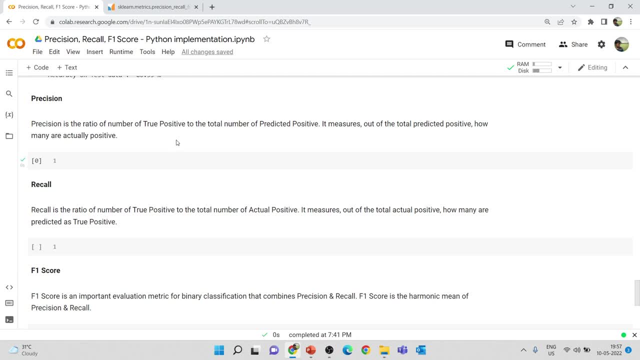 that case, a person doesn't have our disease, but our model is telling that that person may have our disease. so that is what we call as false positive. so this is how it corresponds to the true negatives and false negative and so on. so you get a clear understanding of these terms if you watch the previous. 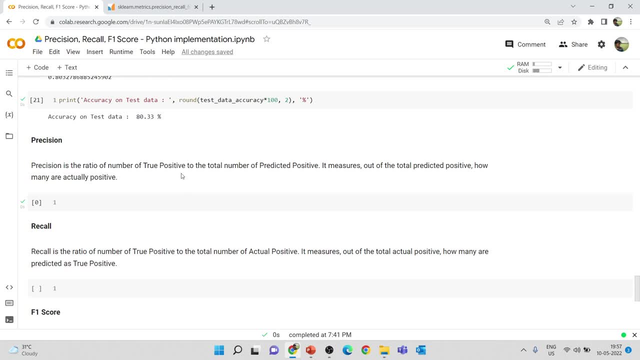 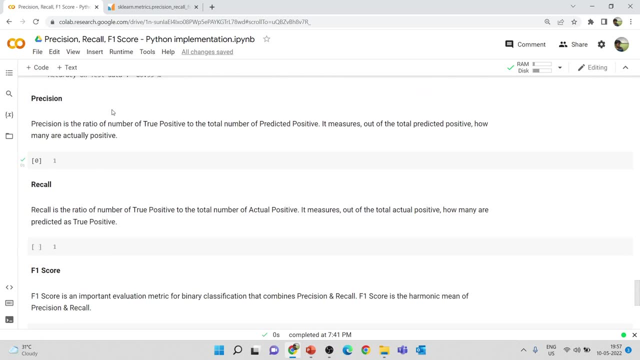 videos. okay, so now we have this accuracy score, details and so on, and now let's try to understand how we can calculate these three metrics: precision, the recall and a fun score. and other important thing is this is used only in the case of binary classification problem. so binary classifications means we are 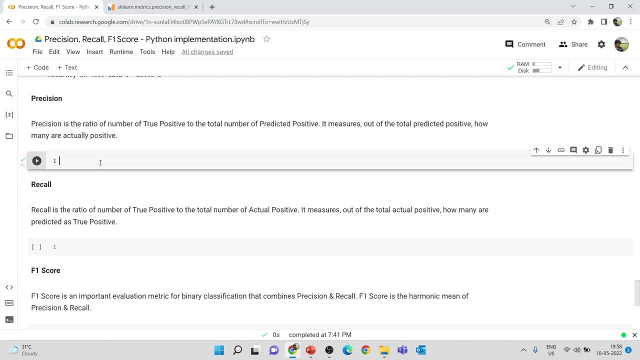 classifying the data points into two classes. so in this case it is person with our disease and personal oxidative response. so in this case we have data points in two classes. so in this case it is person with our disease and personal without addresses. the other example is: you know, you can try to predict image. 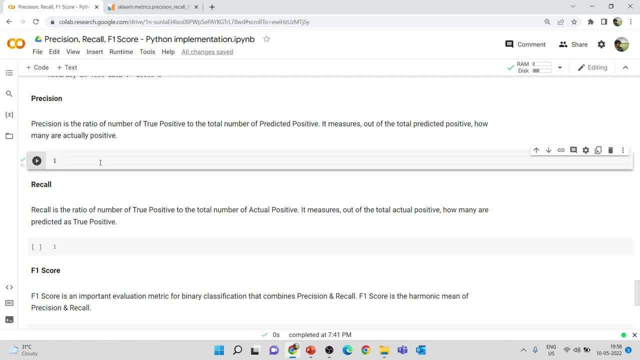 represents a dog or a cat. so there are only two classes, and we are trying to predict among these two classes to which a particular data point belongs to. so that is one thing, and so yeah, let's get started with the coding aspects. so first I'll expose. you know, import this precision score from a scale and so from. 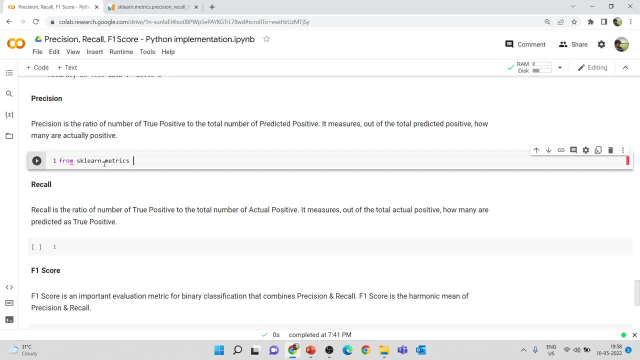 a scale, learn dot matrix. so this is why this is where we have this accuracy score mean absolute error and so on. so all the evaluation metrics will be in this matrix module of a scale. and okay, so from a scale and dot matrix, let's import precision score, the precision score. 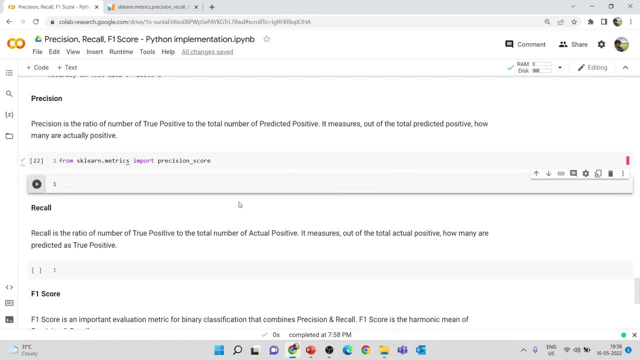 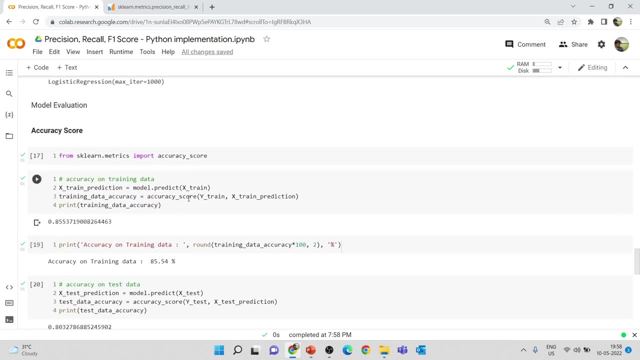 so I'll run this one. and now we have to pass the true value and the values predicted by our model. so we have already did those things in this step. so if you don't understand this, as I have told you, please watch that accuracy score video and the. 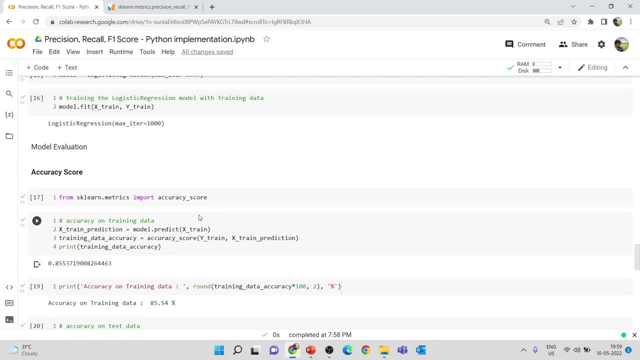 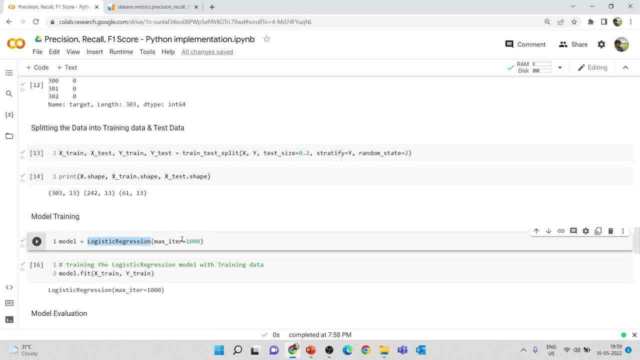 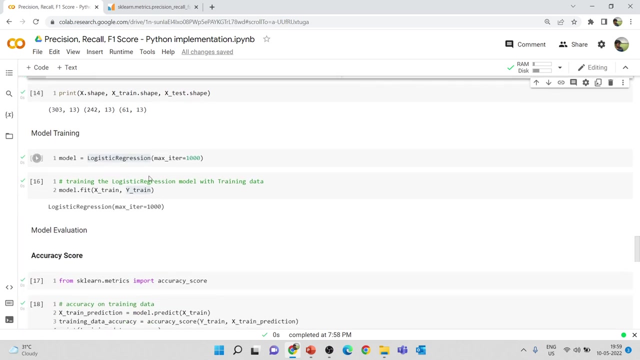 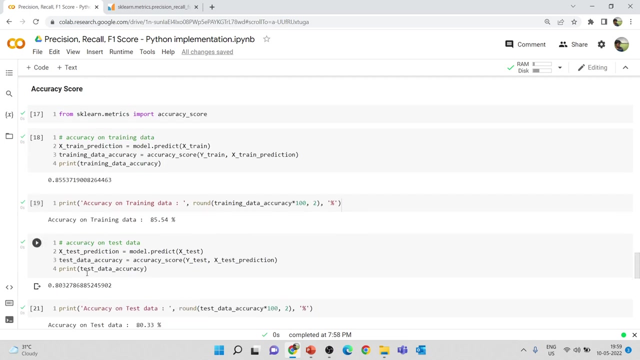 R, o, o, o, o, o o percentage. so we have split at the data. we have trained our model using and this training data. so this is the accuracy on the training data and this is accuracy on test data. so here extreme prediction is the values predicted by your model. 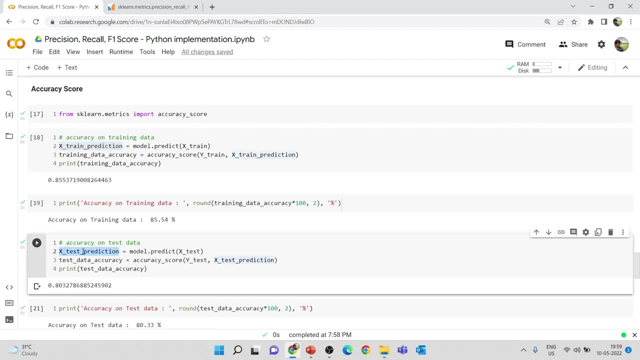 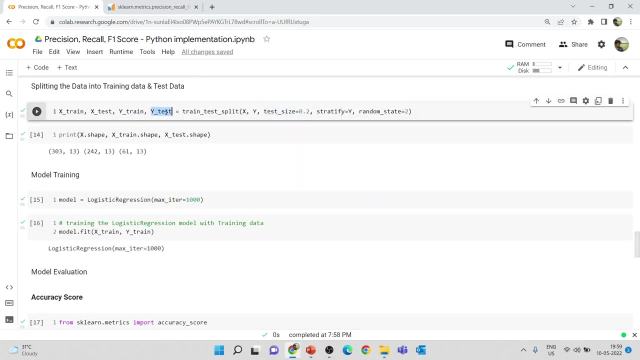 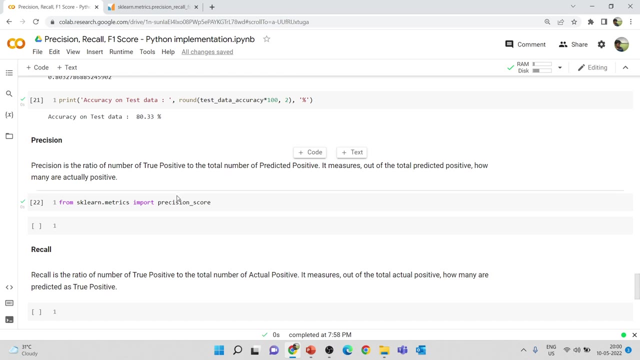 for the training data and the X test prediction, is the values predicted by your model for the test data. okay, and the true values are your Y train and Y test. okay, so this is the true values for training data. this is the true labels for your test data, so we have to pass these. you know four things individually. 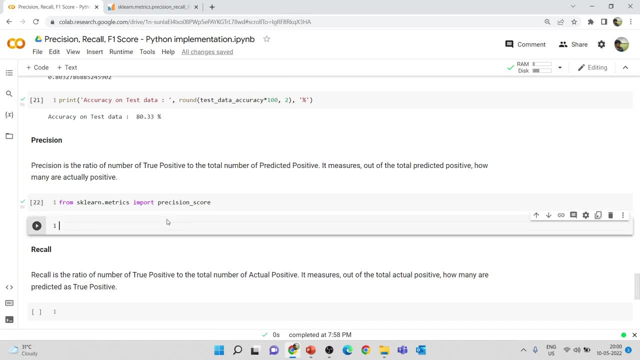 in order to calculate this precision score, recall, a reference score, so whatever we need. okay, so here I will make a comment as precision for training data: precision for training data predictions. so we are. so we will be finding this accuracy score, as well as precision, recall and reference score for. 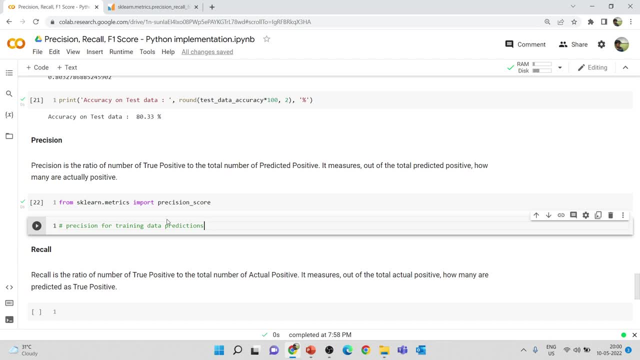 both training data and test data, because then only we know whether our model is working. overfitted. overfitting means in that case your model the overland, and when that happens you will get good accuracy score, good precision value, only on the training data, but your model performs really bad in your test data. so that is. 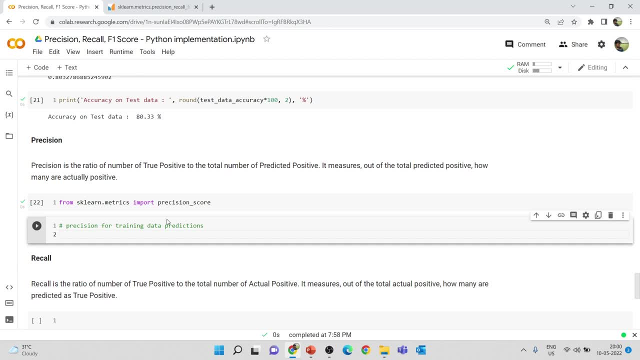 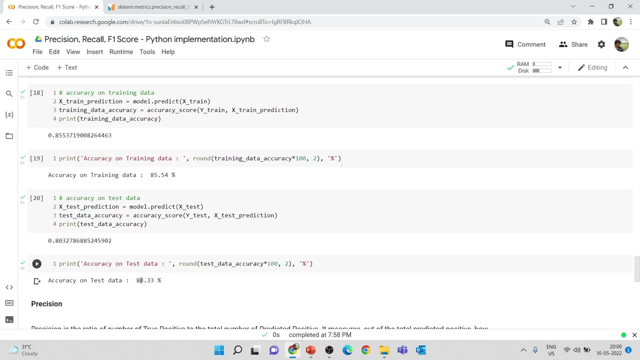 what we call as overfitting. so the main idea is to make sure that the training data accuracy and test data accuracy are close to each other. in this case, the training data accuracy is eighty five point five, four percentage and the test data is eighty point three percentage, so we know that it is almost close, so there. 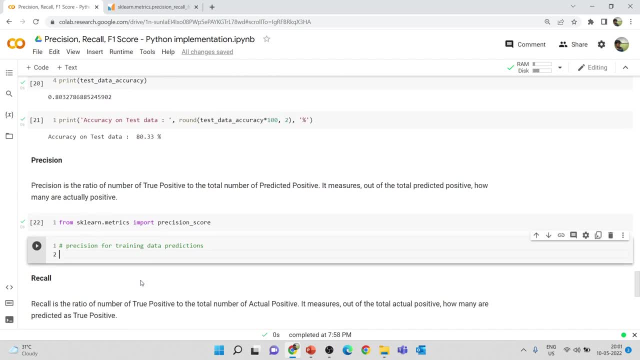 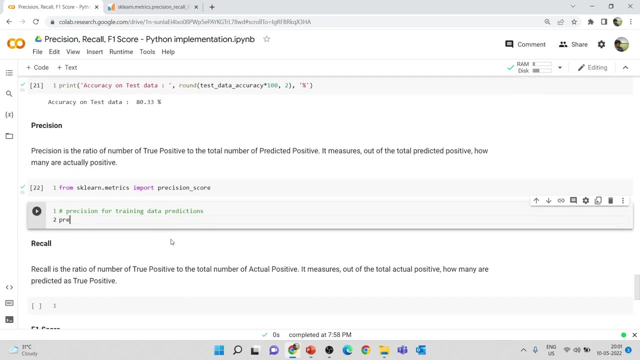 is, no overfitting is happening and the model is working well in in fitting. as for fitting and under fitting aspects, we don't have any issues. so now we have this precision for training data prediction, and here I'll create a variable as precision frame. so this is the precision value for the training. 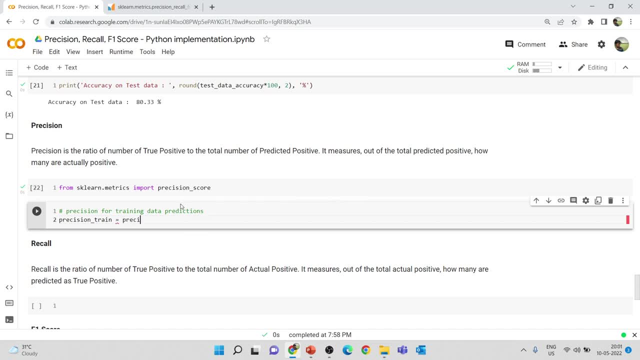 data, and here we have to use this function: precision score. so precision score, and here we have to pass that. we have to pass two parameters: one is the true labels and the other one is the values predicted by your model, which is your extreme prediction. so this is just. 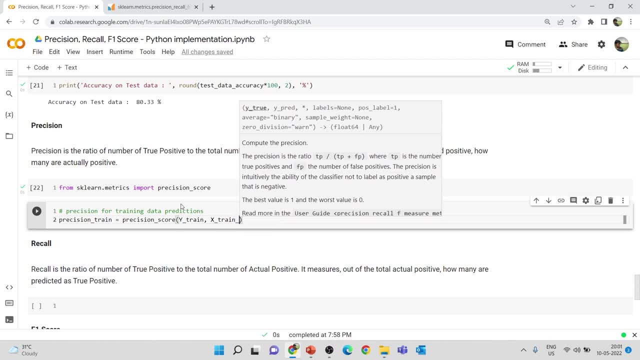 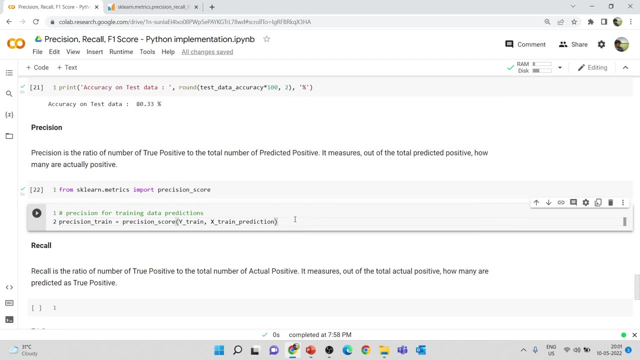 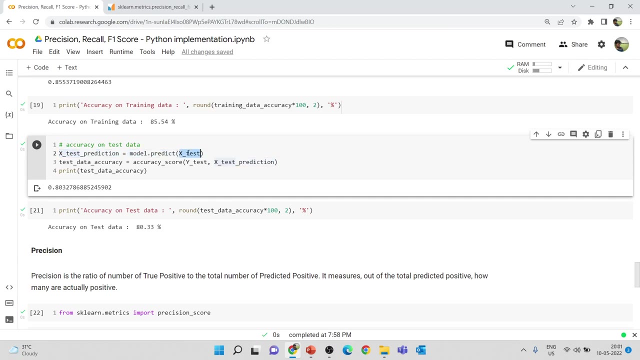 sorry, so it's extreme prediction. okay. so here this is just a similar to the accuracy score that we are calculating, so it is like very similar to it. so this is the values predicted by your model. as you can see, model dot predict X test, so we are passing the test. 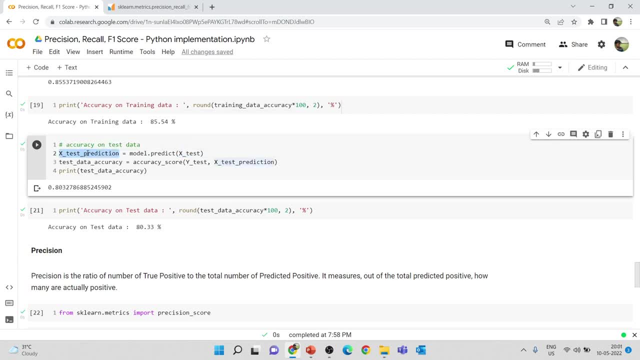 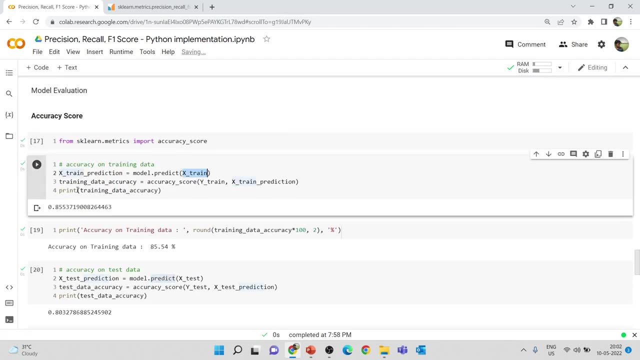 data points features and we are predicting the labels and we are storing this in X test prediction. so this is when we are predicting it. so this is what is data- the same thing we have done for training data as well. so we just have to follow these steps. so I am just giving those errors: precision underscore, train precision. 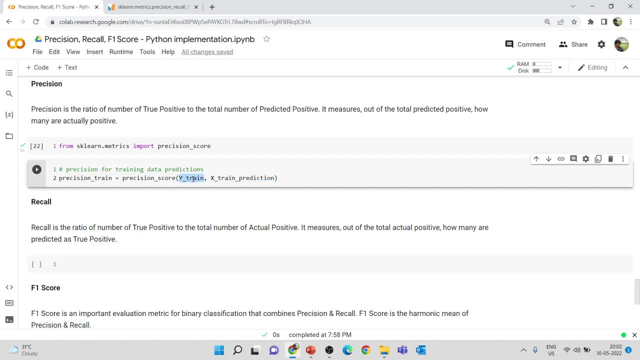 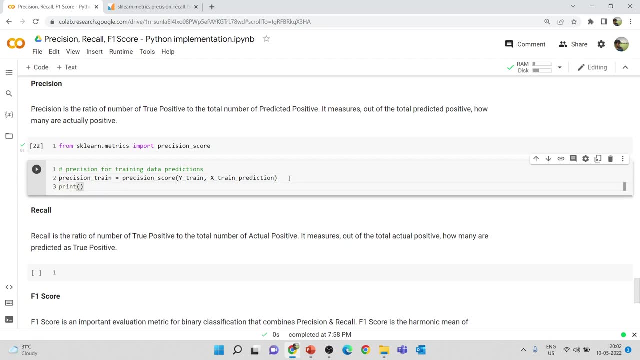 score. so why train, index train. so this is my true labels for my training data and these are the labels predicted by my model. okay, and here let's print training data precision. okay, so training data precision is equal to precision trained. so here we are creating a variable and here we are here using this precision score, which 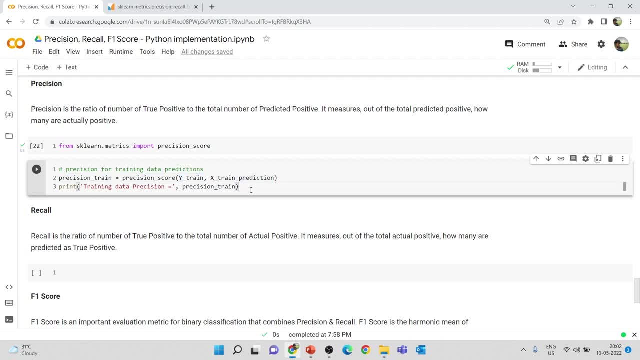 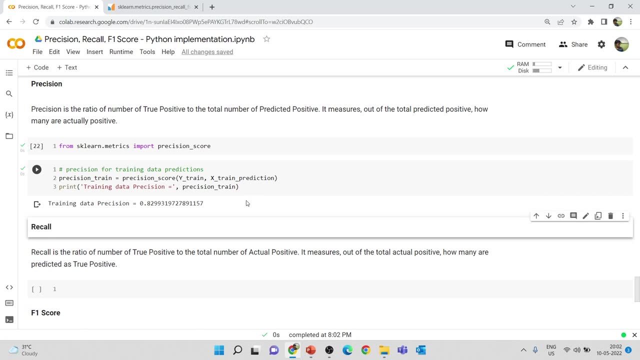 will calculate this score using the true labels and the labels predictedable in mind by our model. okay, so this will give us a value on. this value will range between zero and one, one being your, you know all the values are actually� Goswami, so that what it means. so it ranges from zero and one, so if you want, you can convert. 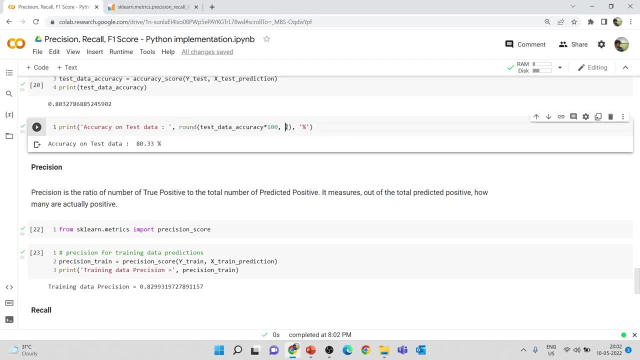 this into percentage, as we have done here, so you can round this to two decimal points and you can include a percentage symbol and multiply it with aajes skin- yeah, we move as you can see that it changes港. multiply with 100, so it basically converts this value, which ranges between 0 to 1, to a percentage. 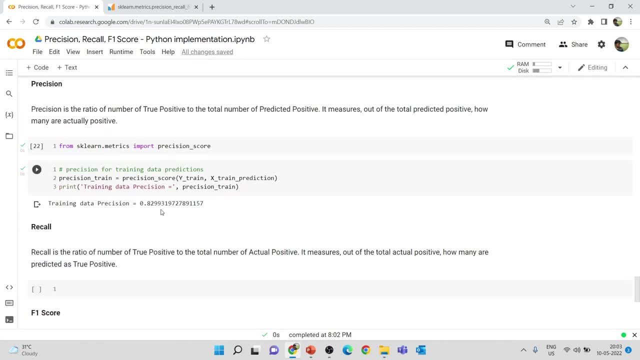 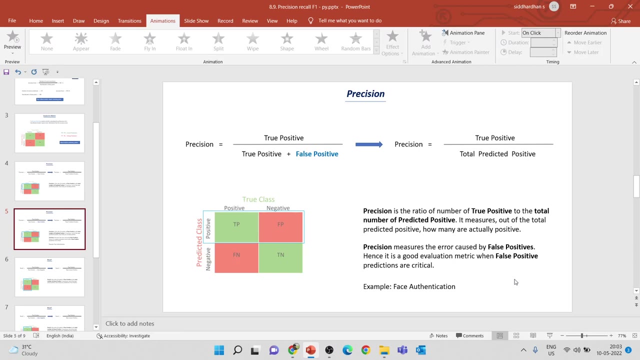 value. okay, so in this case the percentage is 82.9. okay, so almost 83 percentage. so what this 83 percentage means is- you can refer to this definition. so it is the ratio of true positive to the total number of predicted positive. okay, so i have explained this in my- uh, you know- previous. 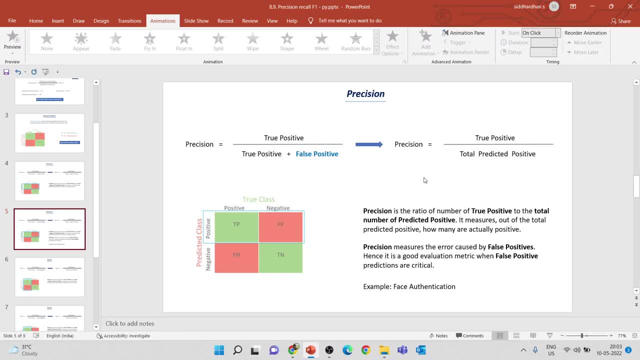 presentation. as you can see, precision is the ratio of the same definition. so it's basically true positive divided by total predicted positive. so out of all the predicted positive, how many are actually truly positive? so in our use case, it's out of all the people who are predicted as those. 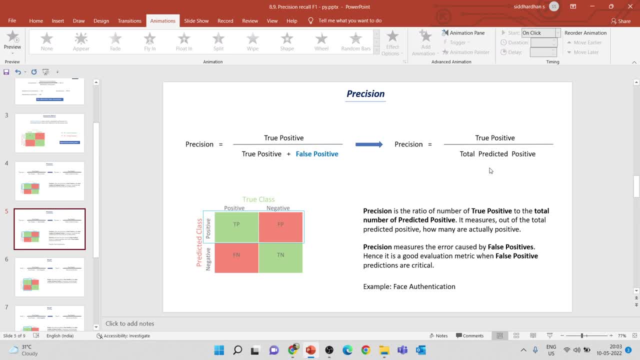 you know, having a disease. let's say that, uh, you know, 100 people are predicted, as you know, with our disease. out of those people, how many are actually having our disease? so that's, that is my true positive. so total predicted positive means all those people who are predicted to be. 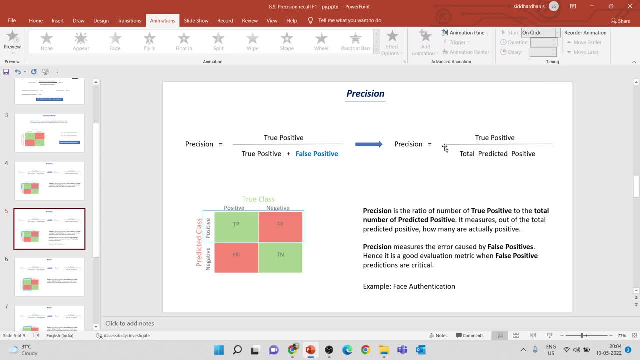 having this are. this is so. that is what precision tells us. so the disadvantage with accuracy is it cannot tell us these details, and these details are very important for us and i have also explained this in the previous videos itself that it measures the error caused by false positive. okay, so total. 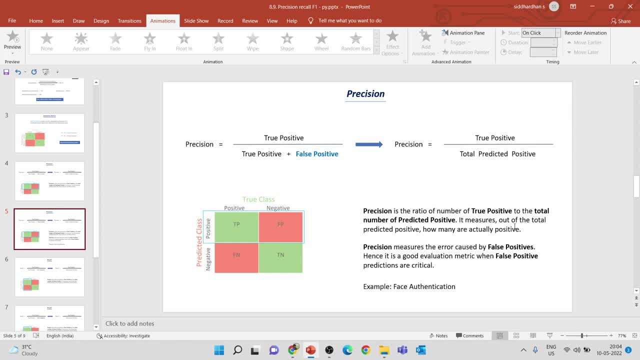 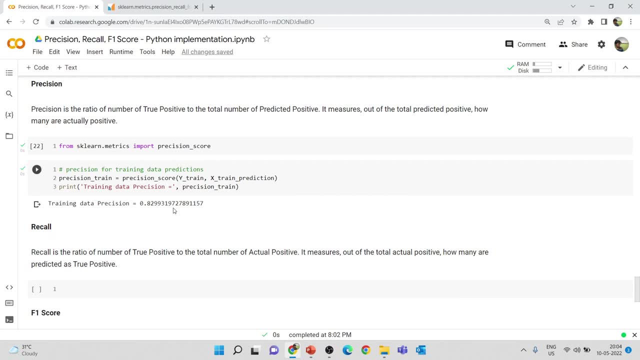 predicted positive is nothing but true positive plus false positive. so it will kind of help us to know the error caused by this false positive. so it will tell us this particular thing. so 82.9 percentage are true positive out of the total predicted positive. now we can, uh, you know, find: 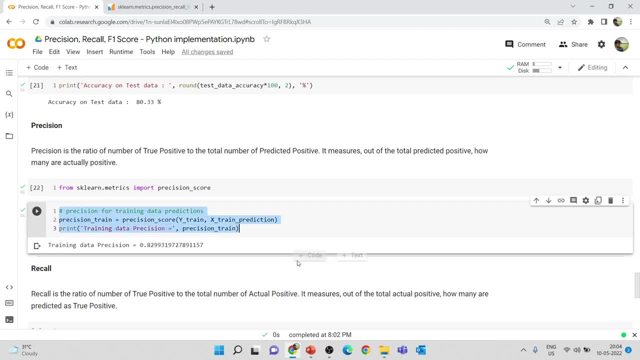 the same for the test data aspect. okay, so i'll just copy this one. so this is for training data precision, and i just paste this code and i'll just change this training to test. okay, so let's name this as precision test, and so here the y train should be replaced as y test and x train prediction. 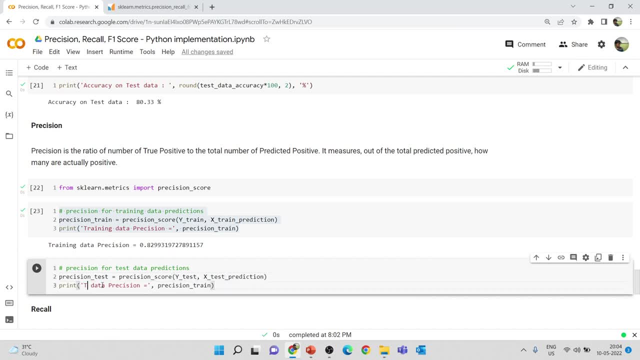 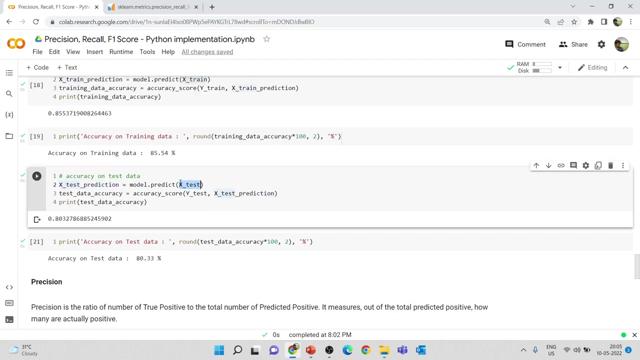 should be replaced as x test prediction. so this is my test: data: precision, the precision test. okay, so i'll just check everything is correct. the precision for test: data prediction, precision test, precision score, y test, x test prediction: okay, so if you see, here x test prediction is nothing but the labels predicted by my model for my test data and here y test, y test. 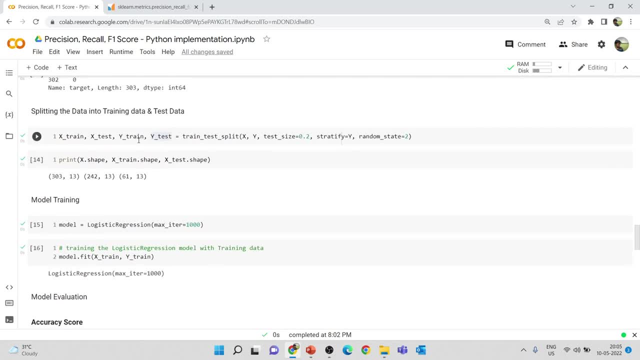 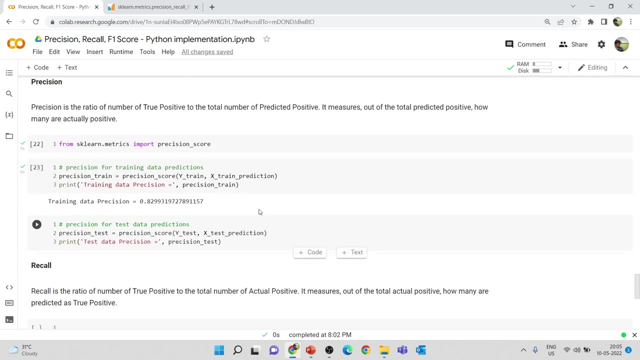 is my true labels for test data which we have scripted using this train test script. so this uh is my test and the values predicted by my model is stored in x test prediction. so, similarly in this case. so we have used y, train and extreme prediction, now we have to use y test and x test prediction. 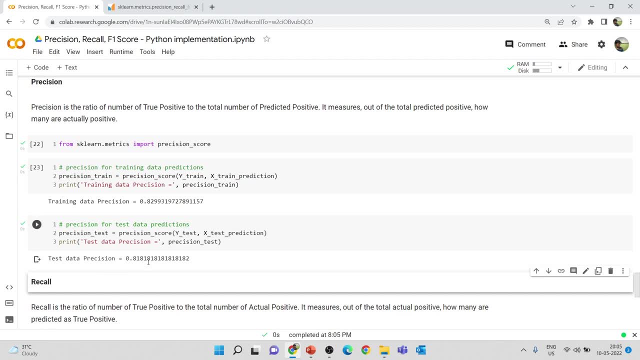 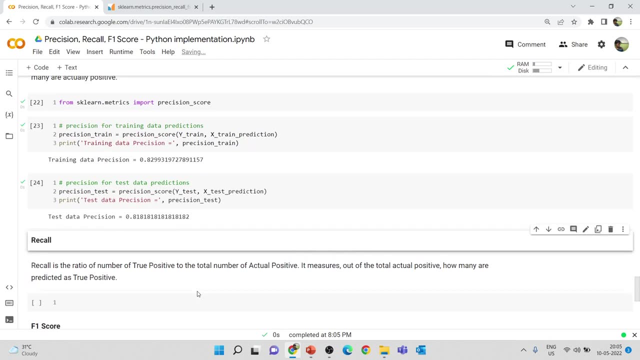 so i'll run this one. so this is my test data prediction, which is like: uh, 0.81 and so almost it's 82 percentage, right? so this is the precision. so recall is so the, you know, implementation is almost the same. so we just have to replace this precision with 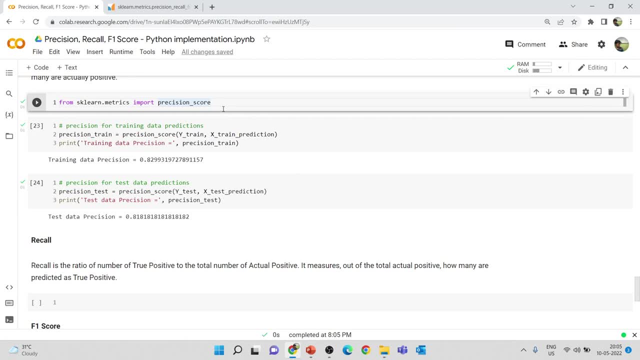 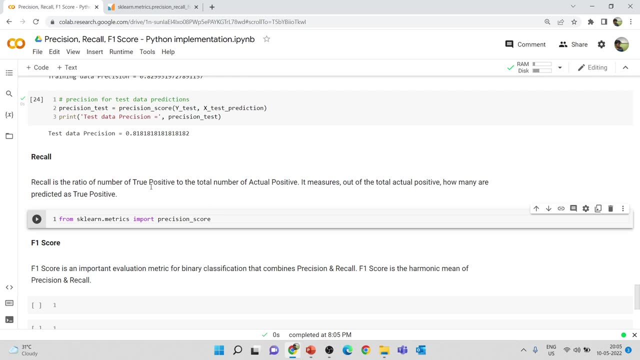 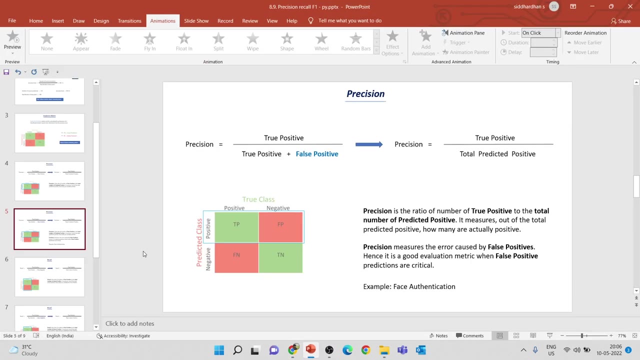 recall and uh, everything else kind of remains the same and this is so. it is not true positive positive. are true positive, false positive. please refer the previous video. okay, so let's go to this recall again. here we have the definition of this recall. i hope you have watched. the previous video. so it basically tells you the ratio of number of true positives to the total number of actual positive. okay, so i'll just open this ppt quickly. so this is what it means. so true positive really be total, actually positive, whereas in the case of- uh, precision we have 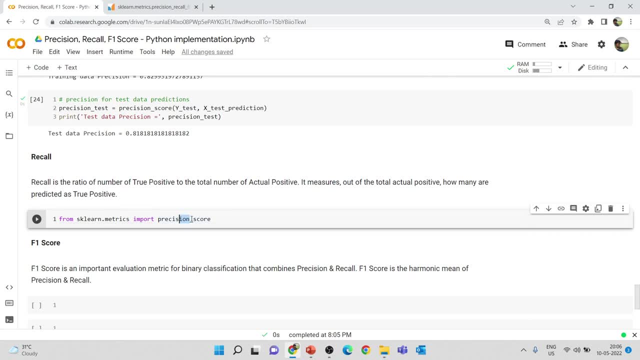 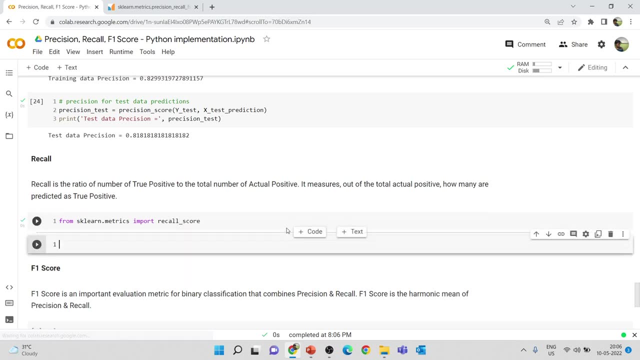 so here we have to change this precision. so in sklearnmetrics itself we have another score called as a recall. so from sklearnmetrics i'm importing this recall score and i'll just copy all these things. i just have to change this precision score to recall score. okay, so i'll. 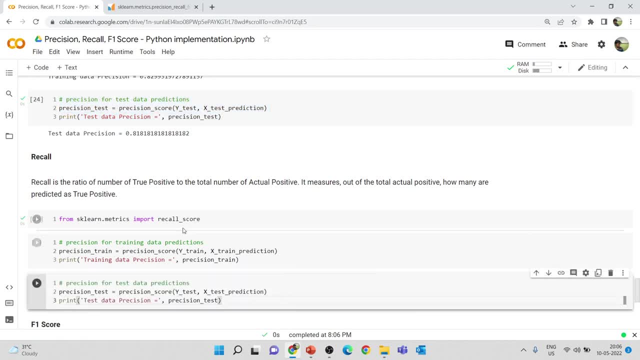 copy this one as well and paste it here. now. let's copy this recall score, put it here. okay, yeah, and so here as well, and i'll just change these things. so this should be my recall recall for training data prediction and let's name this as a recall train. 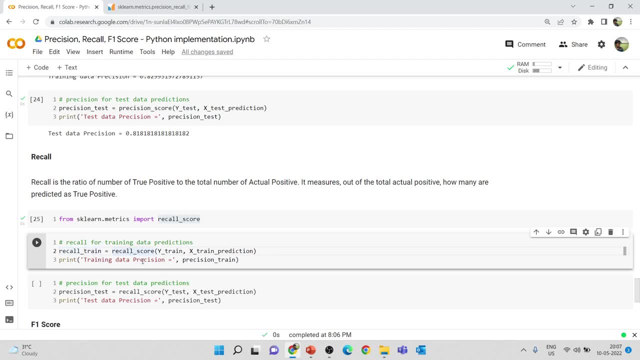 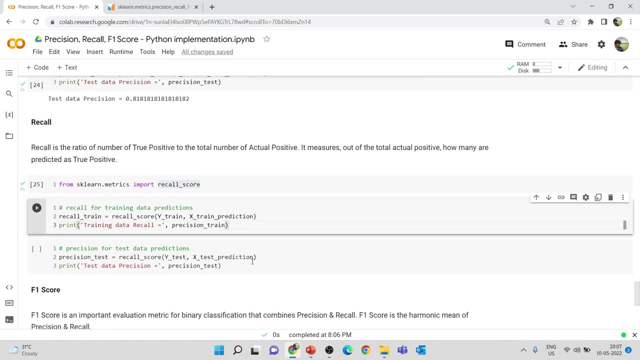 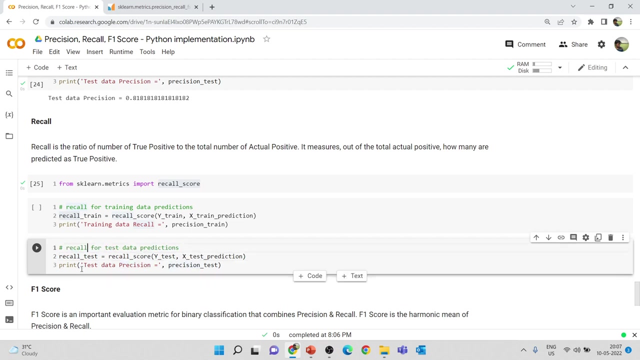 the recall score. so all these parameters, kind of you know, remains the same. so this will be my training data recall. okay, so here we have to replace this. uh, i'll just copy this recall and replace this precision. okay, so this is the recall for test data prediction and this is my test data recall. 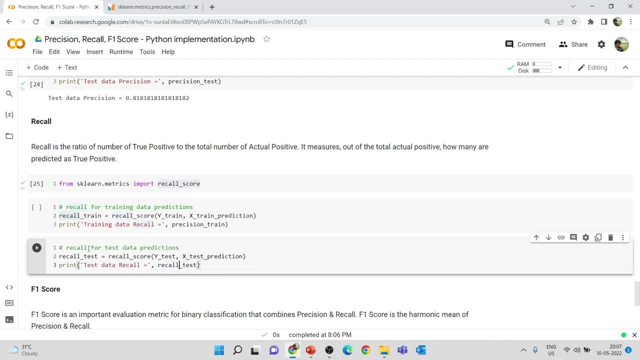 so precision test, so let's run this one. so this is from sklearnmetrics. we are importing recall score, so recall train. so recall of the training data is recall score of y train, which is my true labels and extreme predictions training data recall. okay, so here we have to change this precision train. 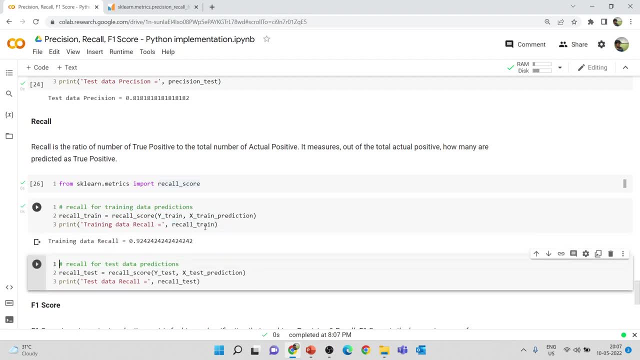 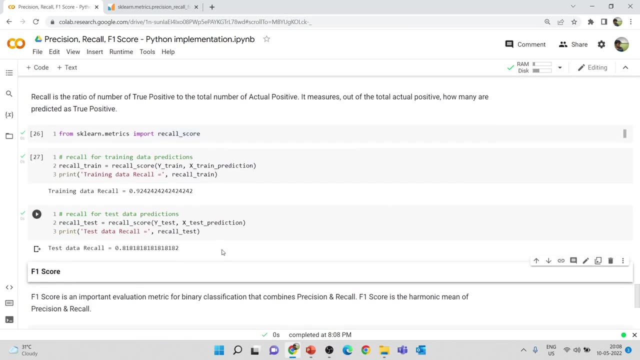 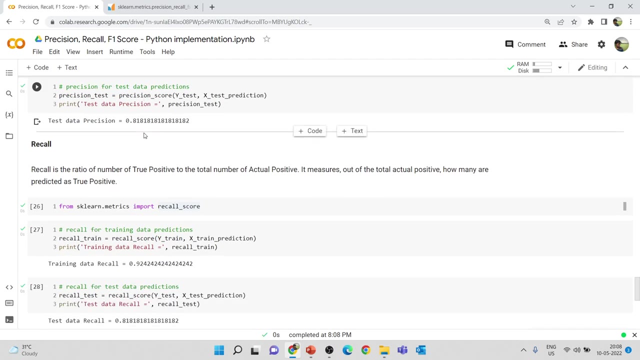 should be replaced with recall train. so this will give you the recall value, which is 92.4 percentage, and for the test data we get the recall as 81.81 percentage. so for this particular data set, i think the uh for the test data, recall, uh, precision and recall kind of remains the same, whereas 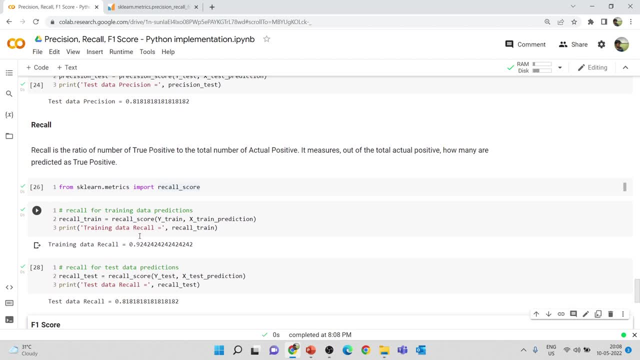 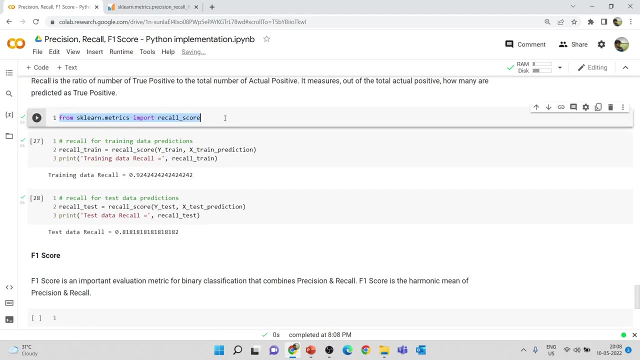 you can see the change in this. uh, you know precision recall for training data values. okay, so this is the same for the f1 score as well. so you just have to rename this. so i'll copy these three cells, if possible. so copy these cells and then paste it here. 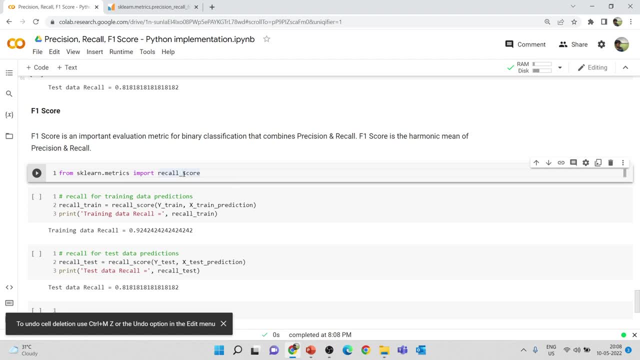 okay, so now we can replace this recall score to f1 score. okay, yeah, so this will be my f1 score. so f1 score is it's kind of a wrapper of these two values. so it will try to find a mean of precision and recall, but it is not a normal mean but a harmonic mean and this is the formula for it. so 2: 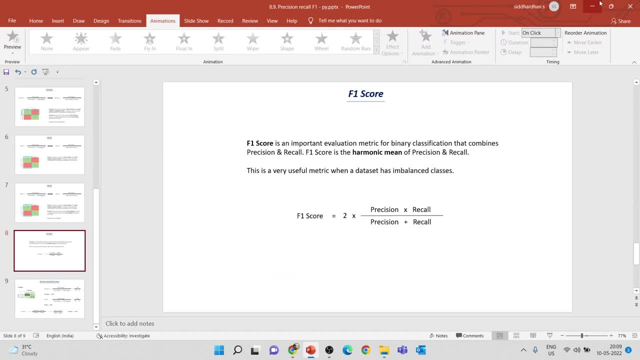 into precision, into recall, divided by precision plus recall. so this is the harmonic mean. if the precision and recall value is the same, in that case you will get the same value as your f1 score. so just like mean. so this is what we call as an harmonic mean. so here we have this f1 score. so 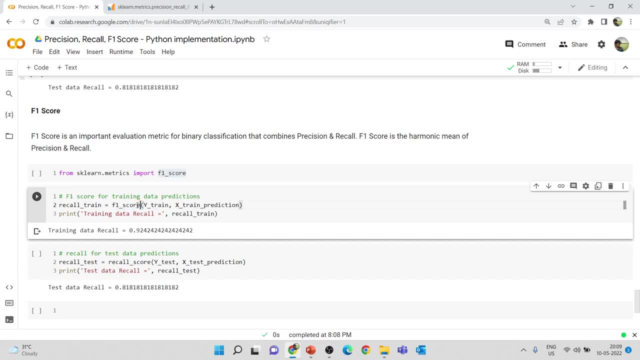 let's replace this: uh, replay, so f1 score. so let me put this recall train as f1 score of train and f1 score. okay, so let's rename this recall test to f1 score test and this should also be renamed to f1 score. so 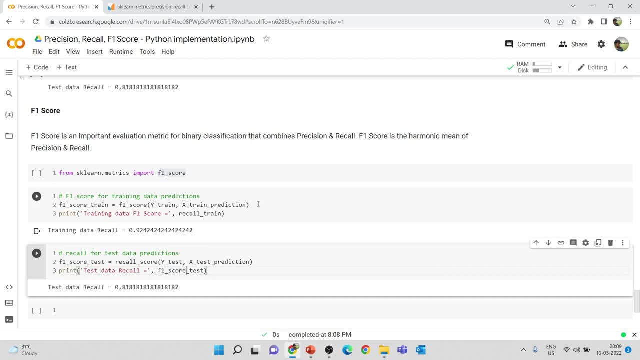 the, as, as we know, that y test, x test prediction and y train extreme prediction- kind of remains the same as they are the parameters on which we are working on. so here let me put this as f1 score for test data prediction. so let's run this one. so here it is: recall train. so it should be replaced. 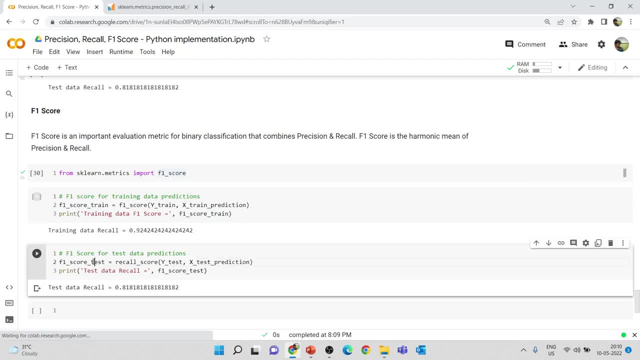 with f1 score train. this should be replaced with: okay, so here it is correct. so here we are calculating the f1 score using this f1 score function and we are storing it in this f1 score train- so white- and index in relation printing training data: f1 score. so this is the same. so this: 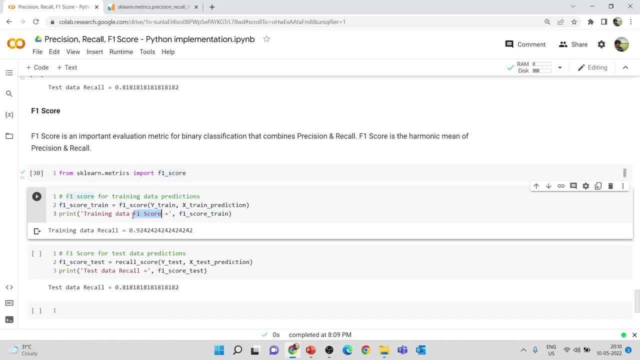 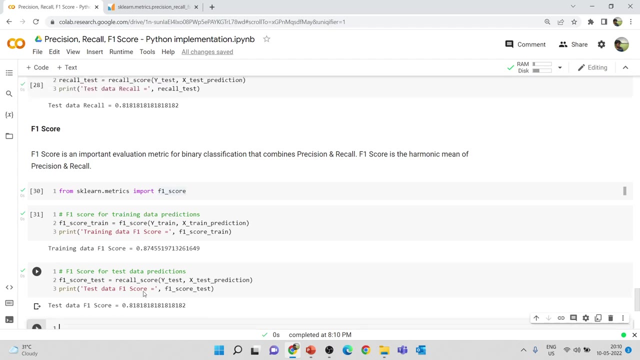 should be training data F1 score and in the next step we have test data F1 score. let's run these two things. so here the training data F1 score is 87.4 percentage and the test data F1 score is 81.8, so almost 82 percentage. so, as you can see, the precision for training data is 82.9 percentage. 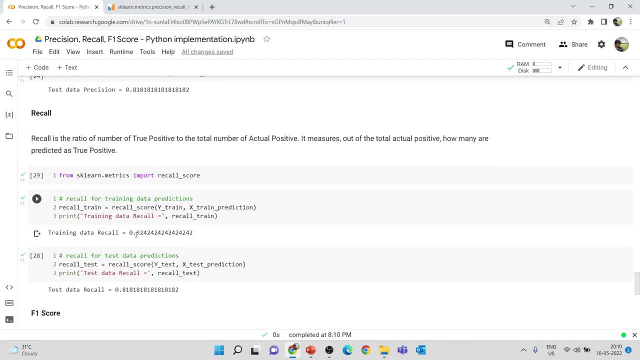 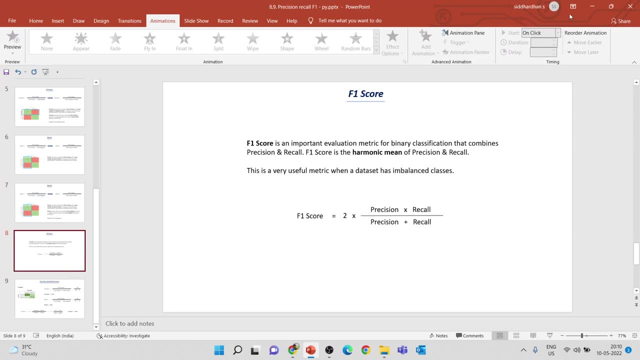 and the recall for training data is 92.4 percentage. so you will get this harmonic mean value to be 87.45 percentage, which we will get you know using this particular formula. okay, as I have told you, in this case precision and recall kind of remains the same for test data, so the F1 score will also. 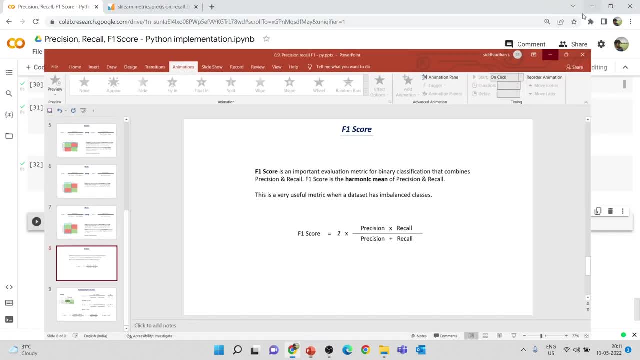 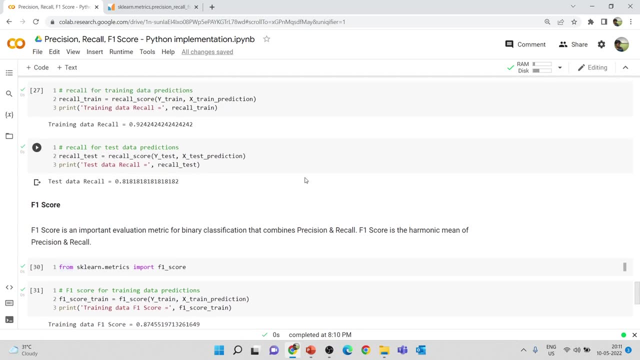 be the same, as it is just another form of a mean. okay, so there is just one more thing that we can do here. so instead of, you know, calculating this precision, if you know recall, and F1 score separately, we can also kind of build a function through which we can, you know, print all these. 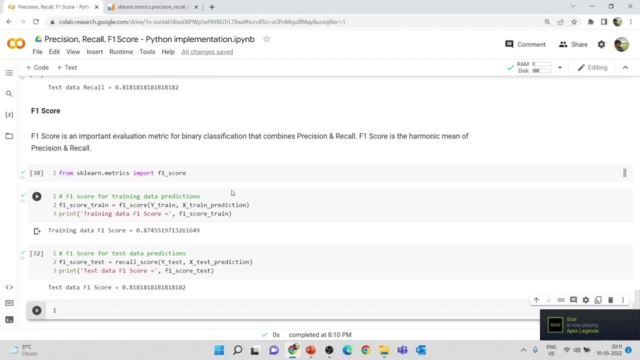 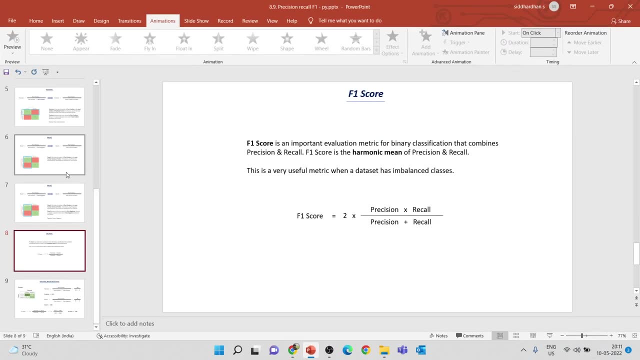 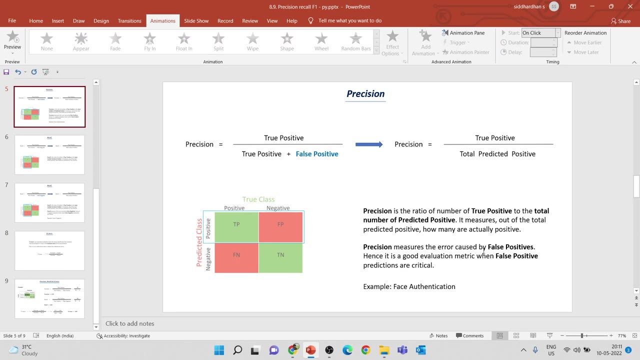 values. so the reason we are kind of calculating this different, you know separately- is we don't need all these three metrics all the time, so they are like, there are like specific advantage to it. so say, for example, in the case of precision, it is very helpful for us in order to you know, in the cases where false positive rate. 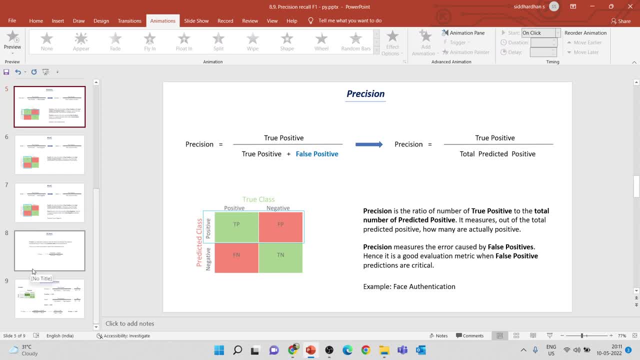 is critical or where we wanted to measure the error caused by false positive, whereas in the case of recall it measures the error caused by false negative. so whenever false negative, you know predictions are critical. in that case we will look into recall more specifically. so that's why I just wanted to show you how you can calculate. 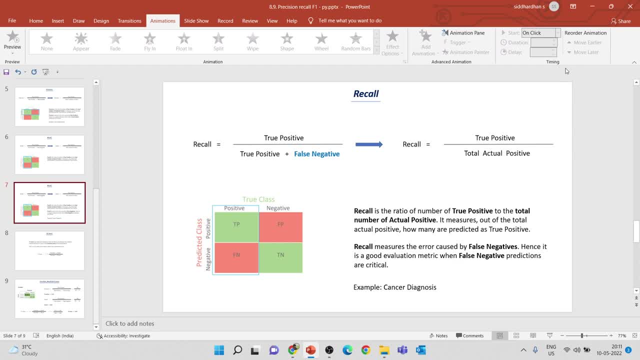 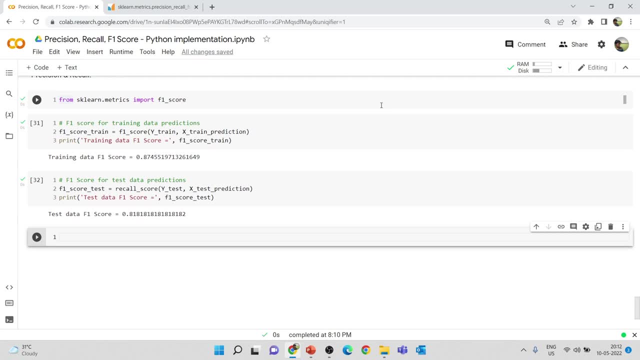 these values separately. so you will understand this with this particular example, if you have seen the previous video where I have explained you why is that critical, why false negative is critical sometimes and why true negative- sorry- why false positive is critical sometimes, so you can understand from that video. now let's just create a small function incorporating all these. 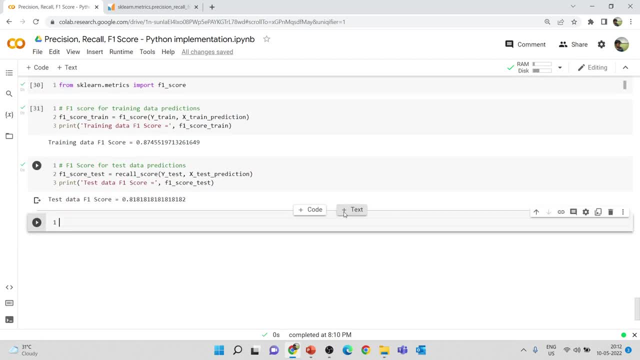 things: precision score, recall score and F1 score, which, will you know, help us to give all this value when we run the cell for one single time. so I'll name this, I'll just put some text here- as precision, recall and F1 score. okay, just a second. so F1 score, and here we are going to create a function. 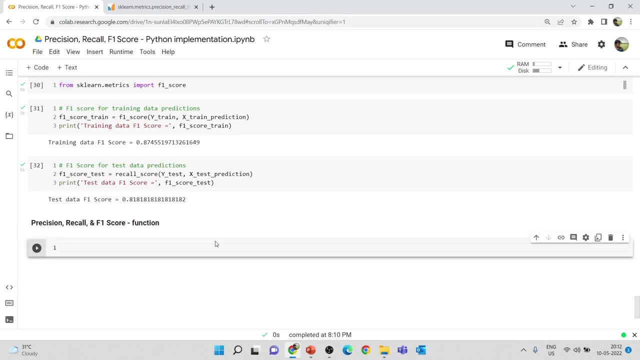 okay, so DEF, which stands for define, and let's name this as precision, recall and F1 score. okay, so this is the function that we are creating, and here we need two parameters. so the first parameter is true labels and the next parameter is our prediction labels, so let's put this as spread. 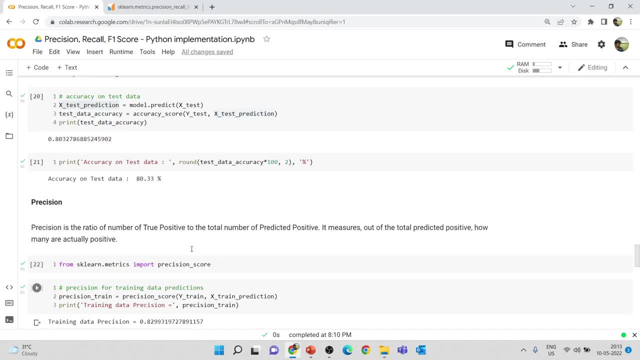 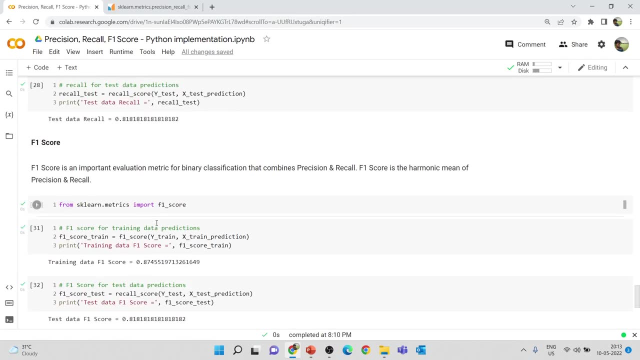 labels. so true labels is the white line, which is the value of the error caused by false negative. so true, negative is the value of the error caused by false negative and true negative is the value of the error caused by false negative. train or y test okay. so what we have here. so, while splitting it, yeah so y train and uh, y test, okay, so. 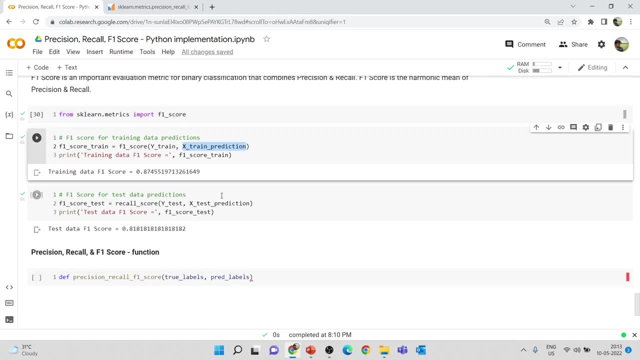 so in this case, the prediction will be your extreme prediction or your excess prediction, so that will be, uh, the two parameters that we have to give here. so here let's create three things. so one is precision, value is equal to. and next let's create um, okay, so let me just complete this. so this will be precision score. so first you have to: 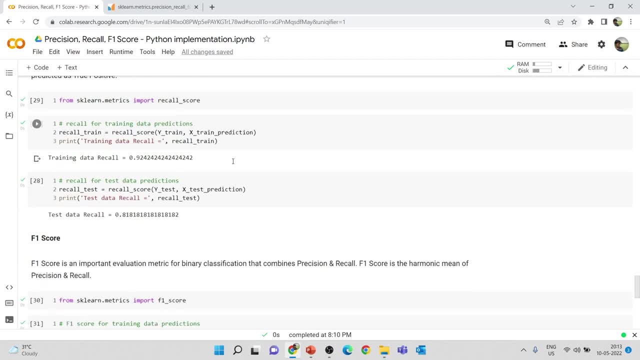 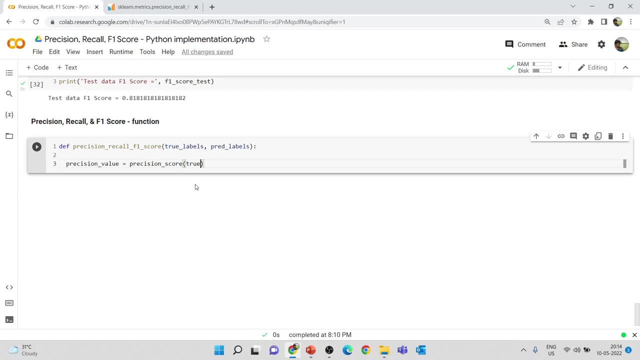 import this. okay, so i have already imported this precision, recall and f1 score separately. so if you are not doing this individually, you need to import these three functions. so precision score. so i have to save two labels, two labels, comma, red labels. okay, and i'll just copy this and we just have to replace this precision with a recall. 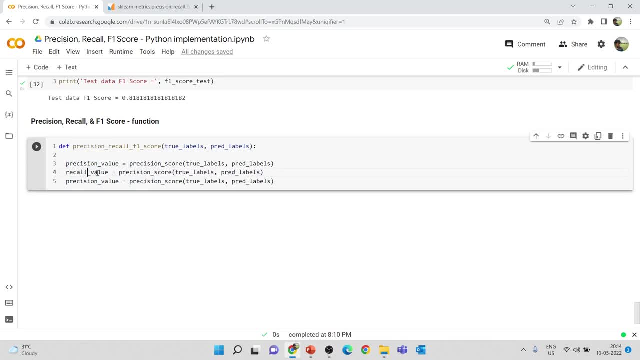 so i will replace this precision with a recall. okay, so this should be my f1 score value. so here also we have to replace those functions recall score and this would be my f1 score. okay. so if you are wondering where this precision score recalls current f1 comes from, as i have 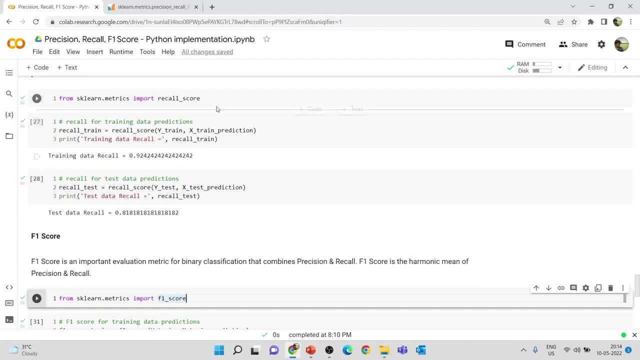 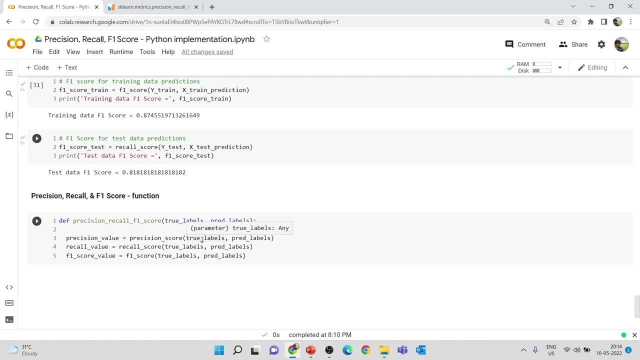 told you we have imported. so we have imported f1 score here and imported uh recall score here and f1 score here. so we are using those functions. so the offer: we know that for all these scores, true labels is the first parameter and prediction label is my second parameter. okay, so which is? 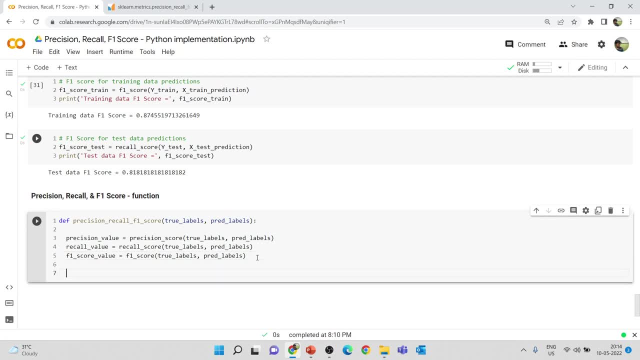 similar to how we carry out this accuracy score. so here i'm going to print three statements. okay, so, if you want, you can return this precision value, recall value and f1 score value. so for this function. so the purpose of this function is to print precision value, recall value and 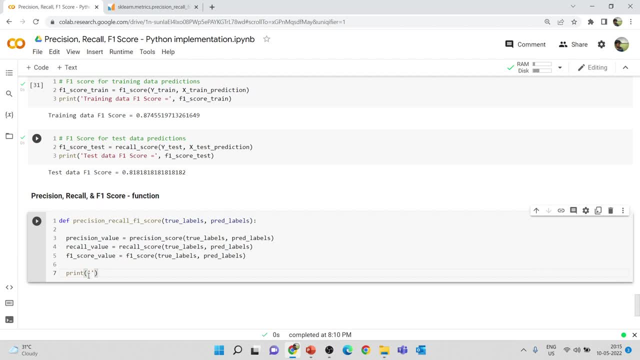 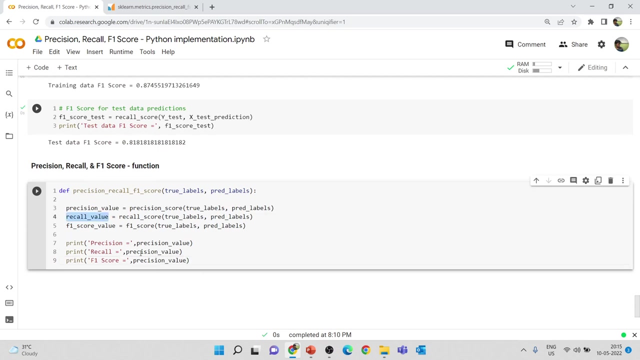 f1 score value. so that is what we are interested in. so i'll put this text here. as precision is equal to uh precision value, let me just copy this, paste it quickly now. we can replace this precision with recall, and here we can replace this with f1 score. okay, so this recall value we have to paste here. so 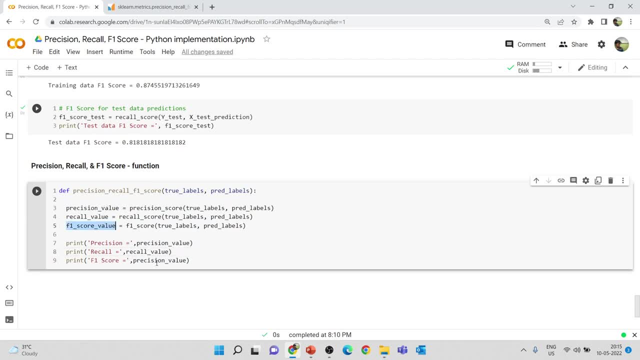 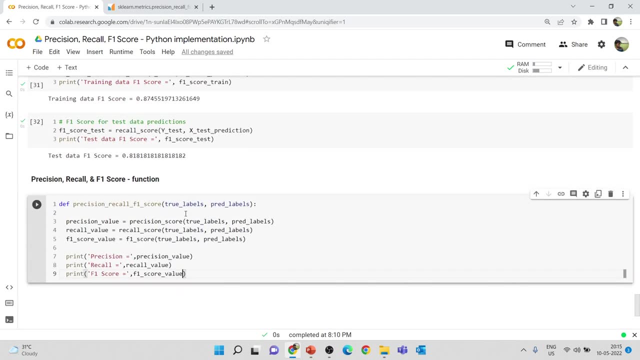 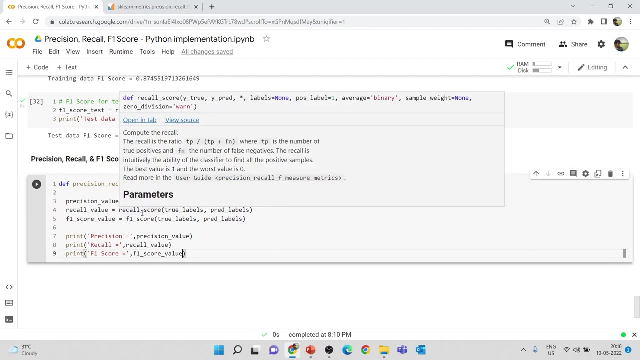 it is just the same thing that we have done before, so i'll show you in a moment. so we are just doing the same thing: finding the precision recall difference- because, instead of doing this in three different steps, we are putting those together in a function which will be, you know, helpful for you in several cases. so instead of doing that, 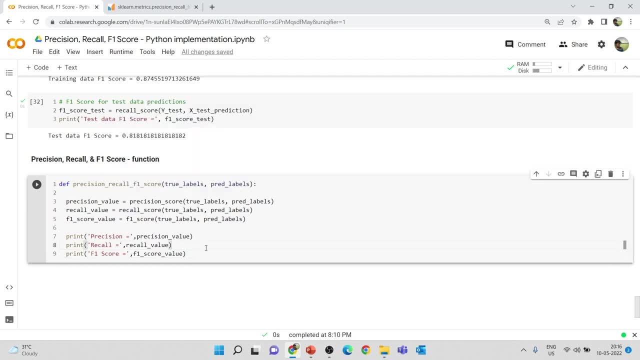 separately. you can set up this function and you can use that multiple times in multiple use cases that you are working on. so that's the idea of this and nothing kind of new to it. so we are creating a function called a precision recall and f1 score, and these are the names of the parameters that we 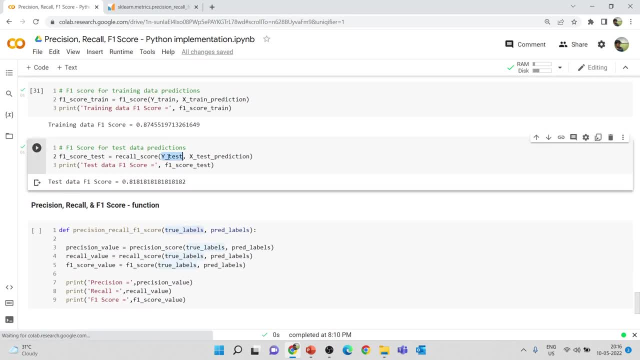 are going to use. so while uh calling this function. so instead of true label we say y test prediction and prediction label x is prediction for training data. we will say this: two labels to be y train and uh prediction label to be extreme prediction. so i'll run this function and now, so we know that. 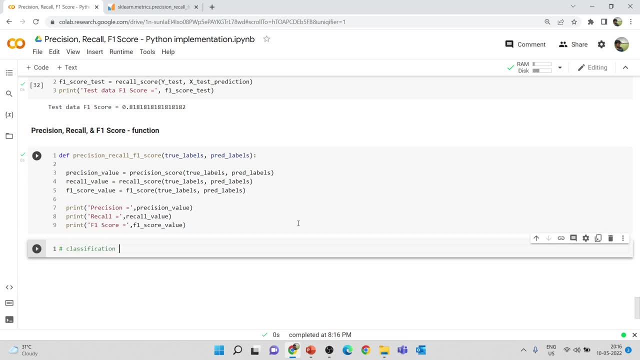 these are classification metrics, right? so i'll just put a text here as classification matrix for training data. so in the end of this video i'll tell you where these scores are. you know very well the classification matrix for training data, so let's name this as: uh, you know. 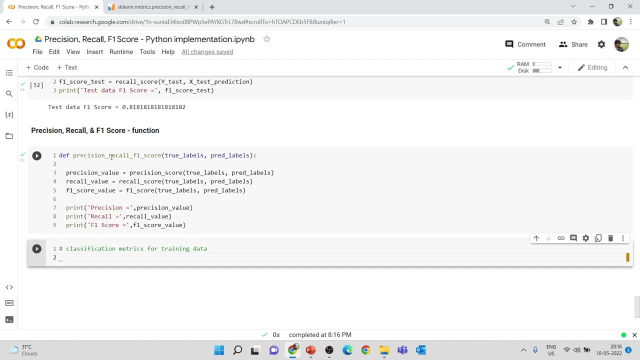 let us call this function, which is my precision recall and f1 score. so once you execute this, so these values will be printed. so this precision value, recall and f1 score value will be calculated and we will print it. okay, so let's pass the parameters which are my. yeah, so this is. 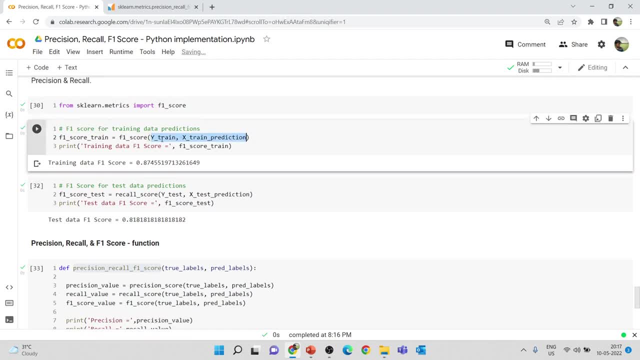 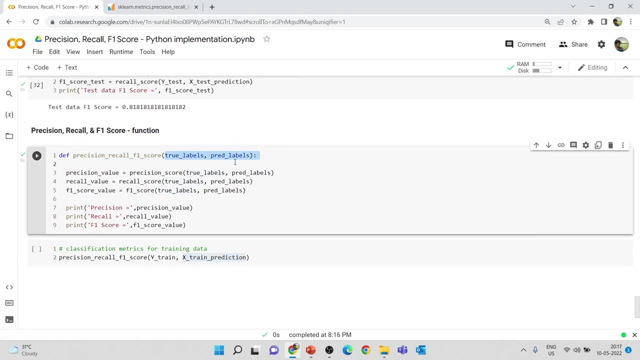 my training data predictions right, so i'll just copy these two things and paste it here. so the reason we are putting these two things is because we have true labels and prediction label as a uh parameters, as we have mentioned here. so i'll run this one, so this will give me my precision. 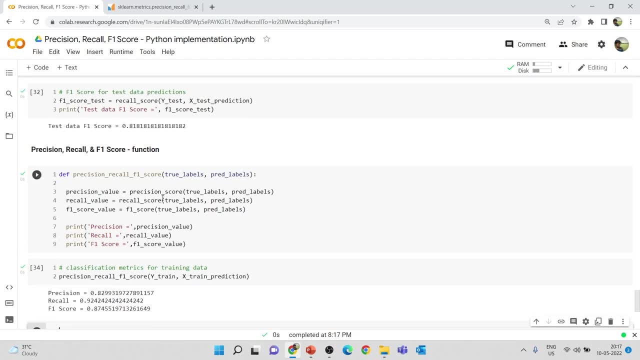 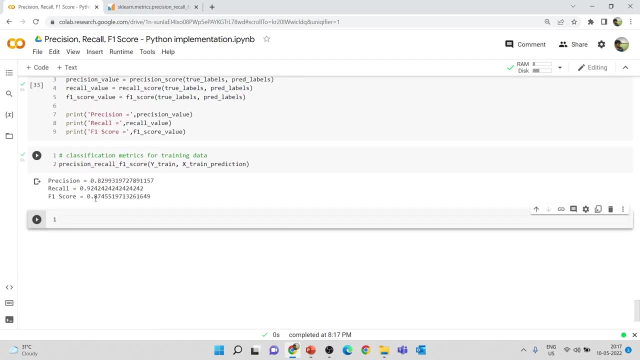 value, recall value and the f1 score value, as you can see here, so which we have got previously. so this is the precision for training data 82.9, which we have got here. so similarly we have got recall value and that's the precision value. so i will just copy this and paste it here. so this is the 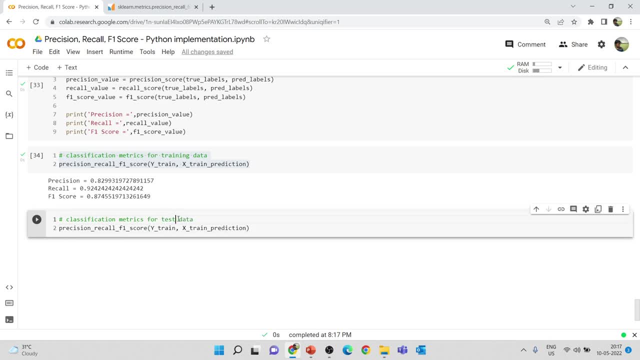 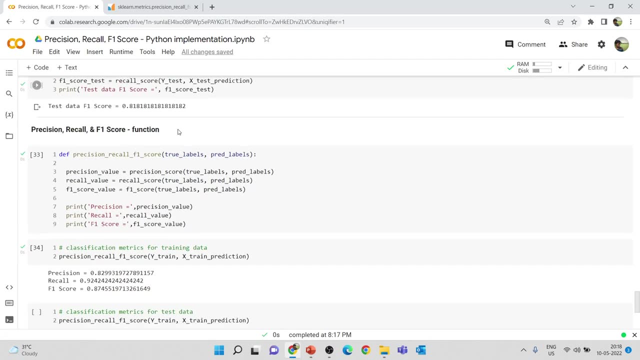 precision value for training data. now we can just copy this, so instead of doing all those things, we just have to call this function. so this is for this data, so we are not doing all the things that we have done here. so we have, you know, calculated this recall and calculated this precision, and so 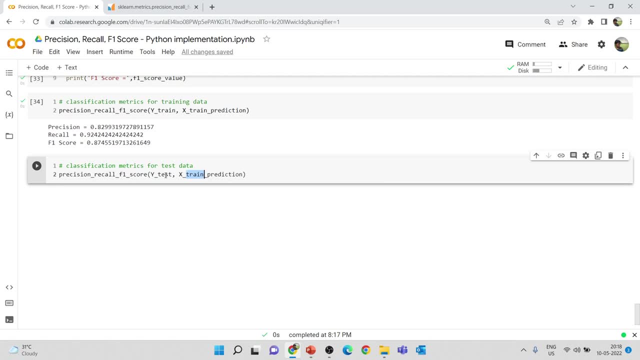 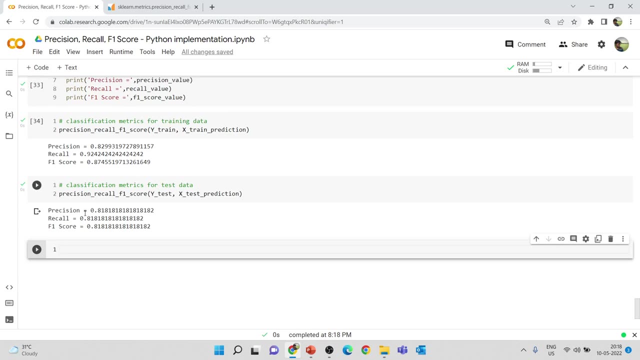 on, right. so you just have to call this function, replace this y train with y test and replace this x test with x test prediction, and these three values will be printed. yeah, so, as i have told you, value to be the same for the test data, as these two values are same, we get the f1 score value. 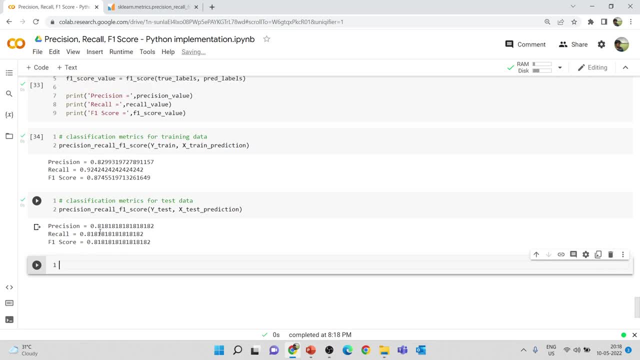 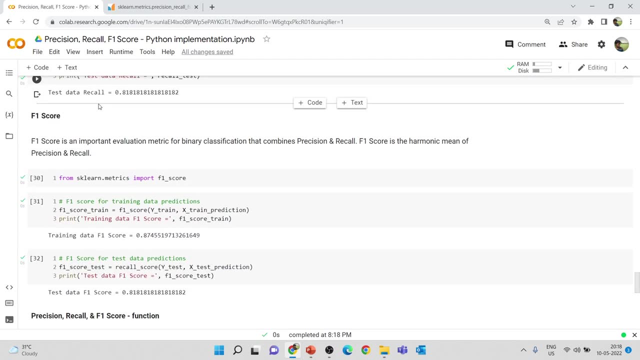 as also the same, as it is an harmonic mean. okay, so this is how you can create a simple function that will give you this precision recall and f1 score, so you can also like kind of find these values individually if you want. so let's say that you are more focused on precision. in that case, you 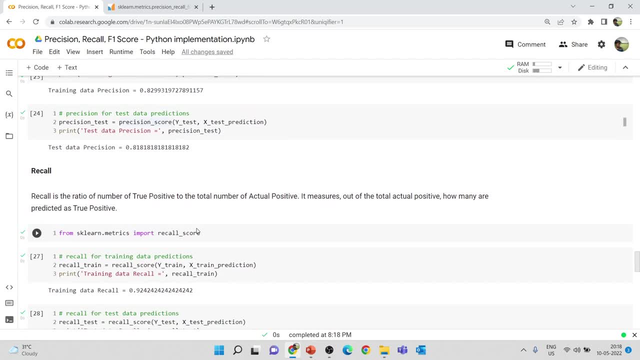 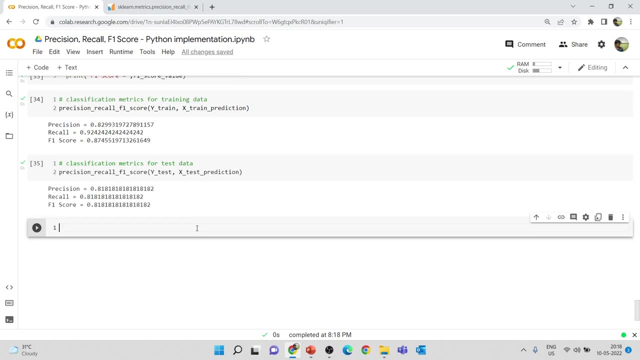 can just import this precision score alone. you don't have to go to recall and f1 score and so on. so this is how you can create a function. okay, so the main, you know aspect in which we use this precision recall and f1 score is when your data set is imbalanced. so that is where these are like. 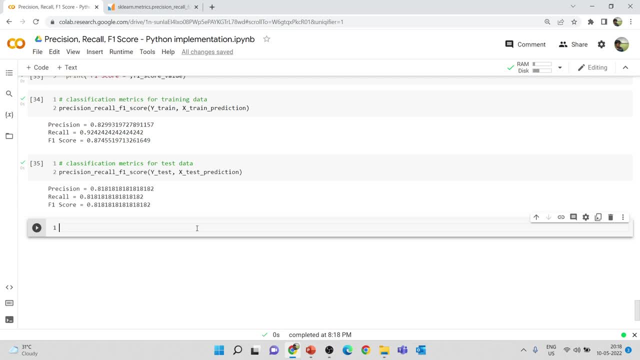 very helpful because accuracy score will be misleading when your data set is imbalanced. let's say that you know we are building a machine learning system or deep learning system that can look at an image and say whether it is a dog or cat. so let's say that we have thousand dog images. 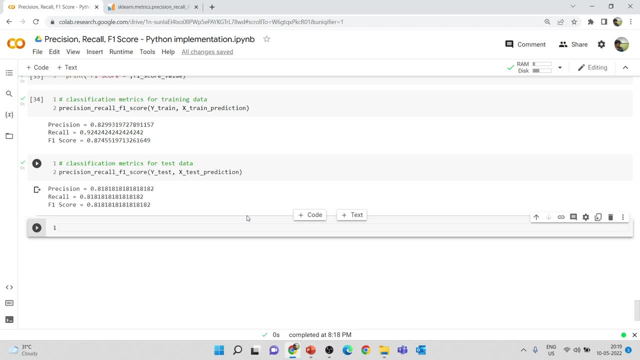 and hundred cat images. so this is what we call as imbalanced data set, because the classes are imbalanced. so in that case you will get a higher accuracy value, but it is not reliable. so i have explained about these things in the previous accuracy score value. so this is where precision recall and f1 score will be helpful for us. so in those cases, 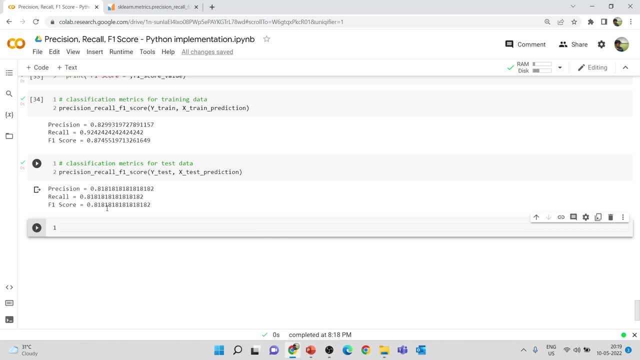 these values will be very less. so that is an indication for us to know that even the accuracy score is high, that the model is not performing well. okay, so that is one main aspect, so you can just remember this or make a note of it. so precision, recall and f1 score are very important. 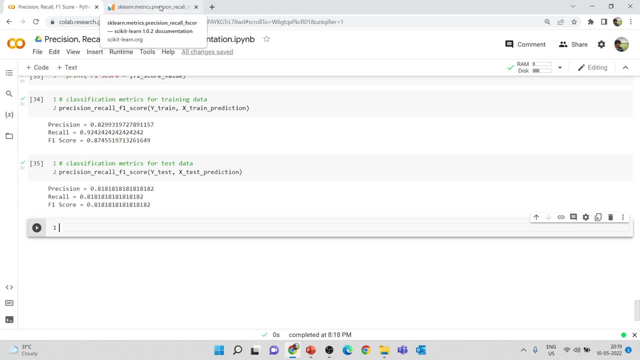 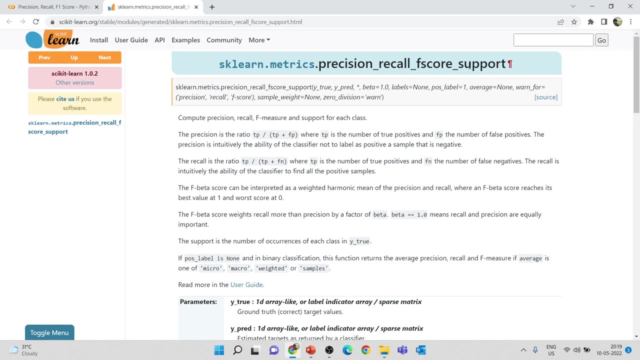 in the case of uh, imbalanced data set- and we also have a function in sklandmetrics which is precision, underscore, recall, underscore, f score, underscore support. so this will give you four values: precision, recall, f1 score and support. the support is another interesting aspect which basically gives you uh, you know, the number of true classes or the number of true prediction. in each class. okay, so, so you know. so. so we are just cal in this case, basically, we have a number of true classes, the number of true prediction in each class. okay, so, so you know. so. so we are just, in this case, basically that is what we have to do. if you want to use that to make a model a. 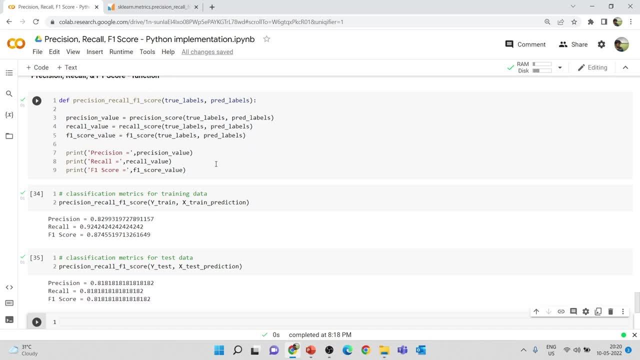 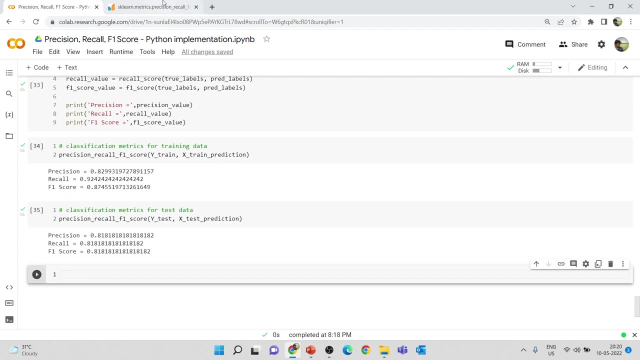 have this art. this is people with artists and people without artists, and we are making predictions right. so in each of these two classes, how many uh correct predictions are made? so that is the support uh metric that we have, but in the case of ml, we mainly focus on precision, recall and f1 score. 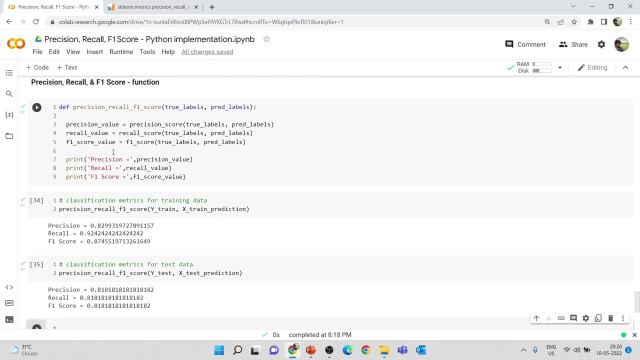 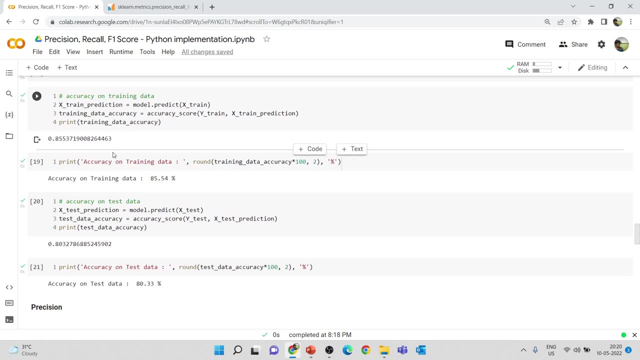 and it is always a good practice, uh, to calculate these three metrics along with the accuracy score as well. so people may, uh, you know, you know, work on some machine learning model trained with data and calculate this accuracy score, but, but it is always a good practice in order to focus on this, 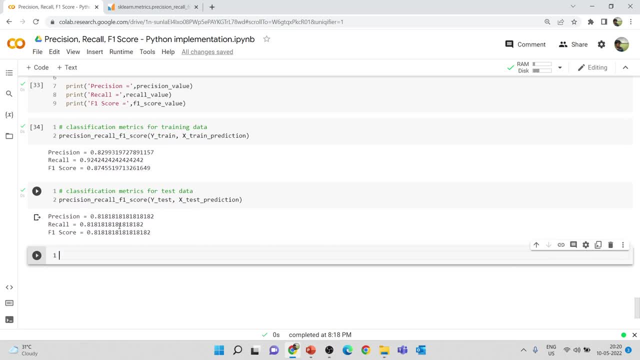 precision three current f1 score as well, and this is a very important concept that you have to know, and this will be asked in central machine learning and data science interviews as well, as this is one of a key evaluation metrics that we have for binary classification problem. so that's it from.